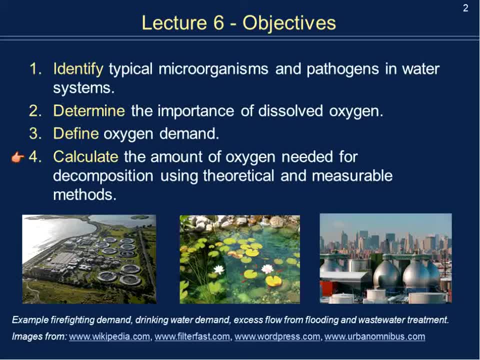 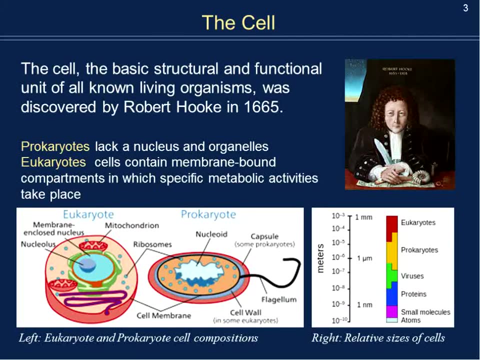 And then, finally, we're going to calculate the amount of oxygen needed to decompose organic matter using either a theoretical or measurable method, And there's multiple measurable methods, but we're going to discuss three of them today. We're going to go back and do a little bit of biology. 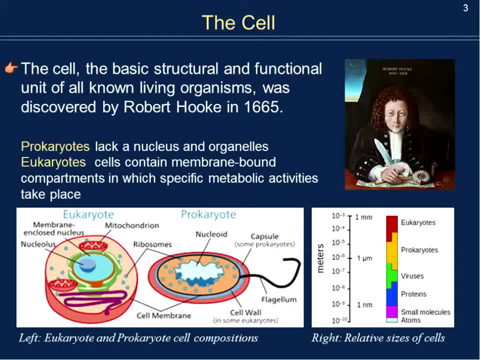 So, again going back, the cell is what's considered the basic structural unit, and this is for all living organisms, And this was discovered by Robert Hooke in 1665.. Now, the two types of structural cells that I'd like to look at are the prokaryote and the eukaryote. 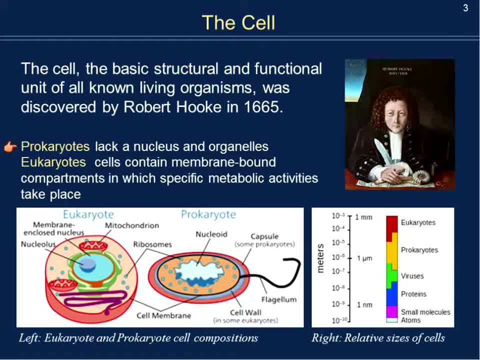 The prokaryote is a very basic organism because it lacks both a nucleus and organized cell structure, which we call it lacks organelles. A prokaryote is essentially just a cell membrane with a general area which is the nucleoid, and everything within the cell performs all of the functions. They're not designated functions. 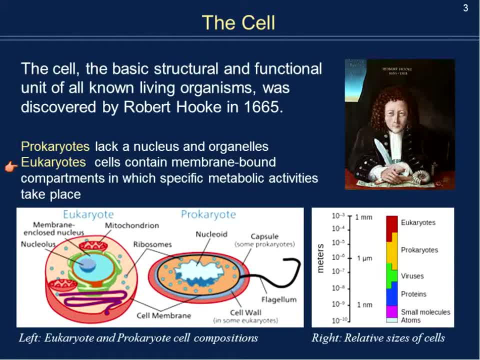 Second, the eukaryote. The eukaryote is different in that it contains what we call membrane-bound compartments, essentially what you would say in your system, such as organs, where they each perform specific metabolic activities. So, just like your heart performs a certain activity versus your digestive tract, versus, say, your lungs, they each have their own function that help you survive. 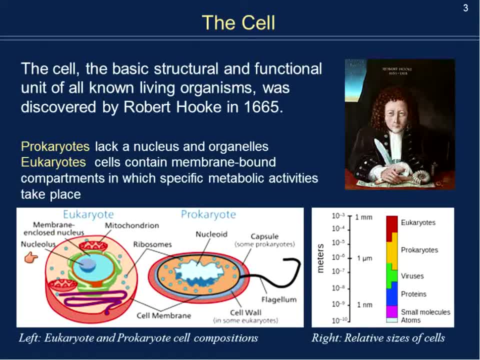 So, if you notice, with a eukaryote, a eukaryote also has a cell membrane but, as you can see, it has a defined nucleus: The nucleolus, the nucleus and the mitochondrion. again, these all serve different functions and they also have ribosomes. 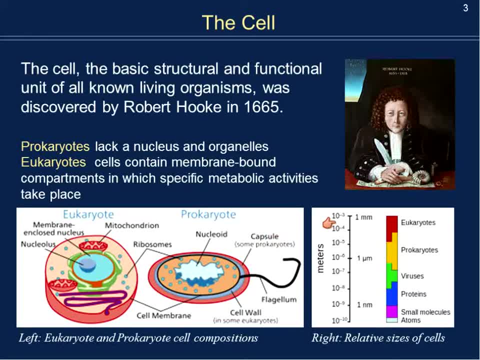 Something to keep in mind: a eukaryote, which is a more complex structure, is approximately one millimeter in length or in diameter. This is something that you can see with the naked eye. So if you ever take out a ruler and look at one millimeter, that's something that you can measure. 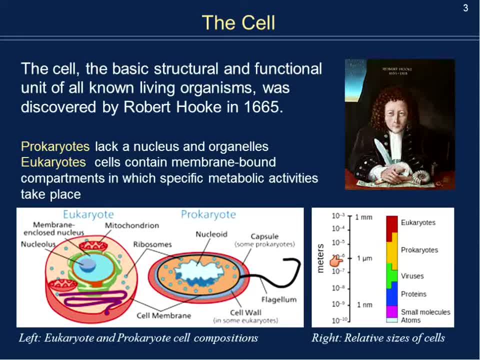 However, a prokaryote is about a thousand times smaller than that, so it's not something that you would see with the naked eye, Neither would you see a virus. So these are three different types of biological systems that we'll be talking about. 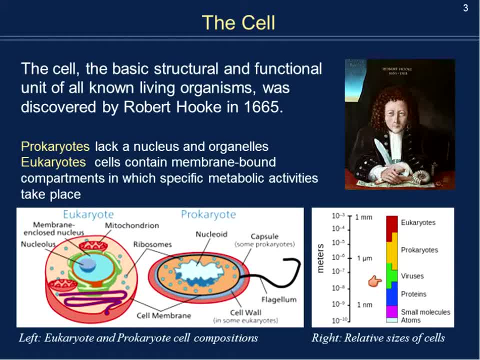 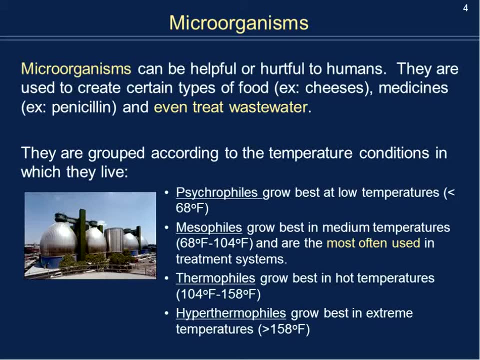 And again, some are what we call good, different types of organisms and others are considered harmful to humans and other pets of animals. So let's talk a little bit more about microorganisms. Microorganisms, like we said, can be helpful or hurtful to humans. 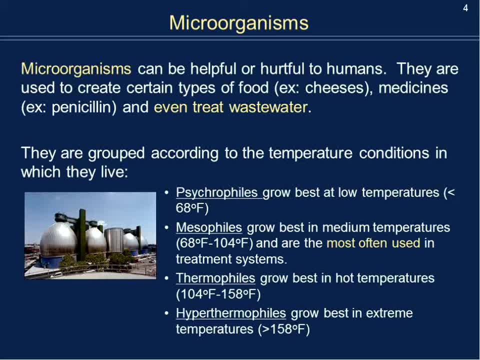 Obviously, the helpful, different type of microorganisms we do want, and those are organisms such as bacteria that move around the body. Microorganisms, like we said, can be helpful or hurtful to humans. Obviously, the helpful, different type of microorganisms we do want, and those are organisms such as bacteria that make cheeses or can then produce medicine such as penicillin. 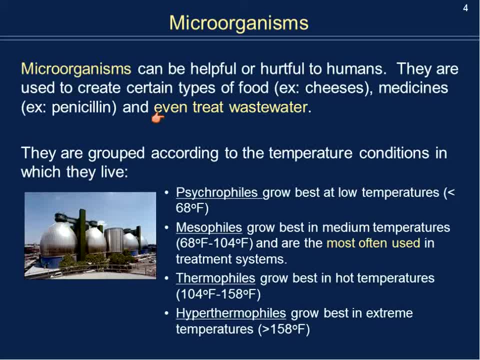 And we can even use helpful organisms to break down and treat our wastewater So we can remove both some of our solid organic material as well as some of the hurtful microorganisms in our wastewater system. But in order to do that- and again, here's an example of what we call a digester. 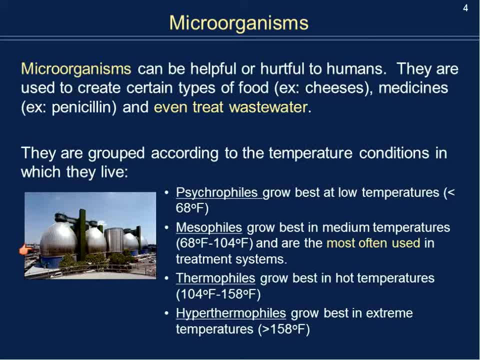 This is, at the Newtown Creek, Very similar, So that's something that we may go see as part of one of our field trips. This is very similar to the digestive tract in a human being And in order to have the system to break down organic material, you often need certain temperature ranges depending on the type of the microorganism. 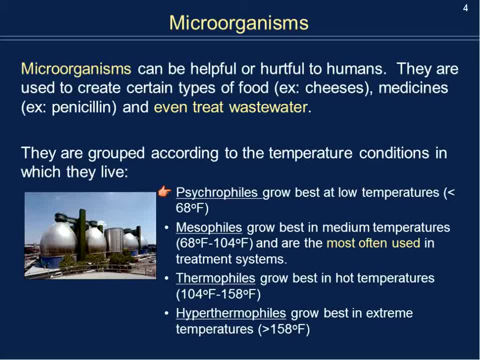 So the first one is called a psychrophil and that grows typically at what we would call lower temperatures, meaning less than 68 degrees Fahrenheit. This would be a temperature range that's much lower than the human system, Where a mesophyll is considered more of a medium temperature range from the 68 to 104 degrees Fahrenheit. 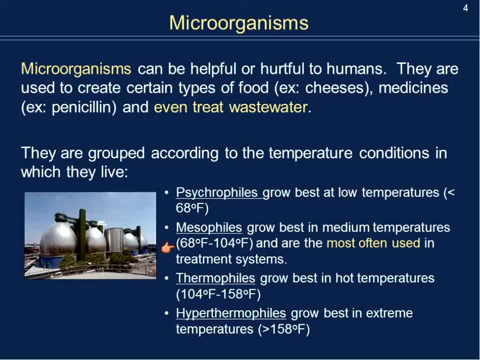 And this is what we would say- mimics more of a human system, And this is most often used when we treat our wastewater. Also, this is the reason why is this range of temperatures- again the 68 to 104, is very natural that we would find in most inhabited areas on the planet. 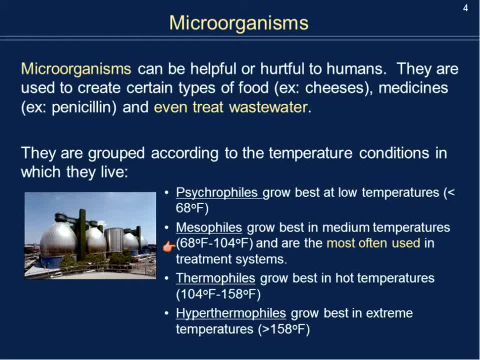 Again, not considering the extremes Such as the poles or maybe some really heavily tropical areas. So this is good because we can use the natural temperature to treat our wastewater and we don't have to heat or cool the system, And that saves energy. 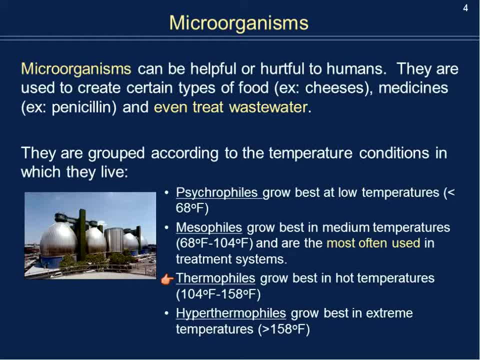 A thermophyll. so when you think of thermo, think of heat. These are typically growing organisms in hotter temperatures, We'll say from 104 to 158.. And then, last but not least, a hypothermophyll. A thermophyll grows best in extreme temperatures greater than 158 degrees Fahrenheit. 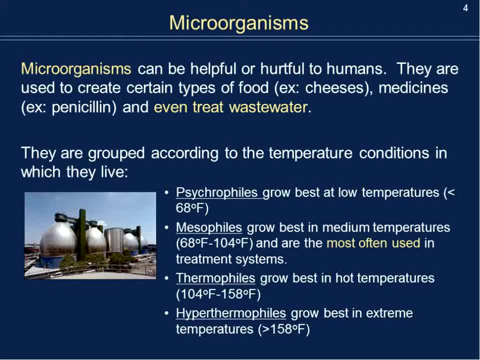 But again, if I can have you just remember for the sake of this, typically we're going to work in the mesophyll range because of the temperature range, Again, just important to note. Now, we talked about good organisms again that help us create foods, medicines and even treat wastewater. 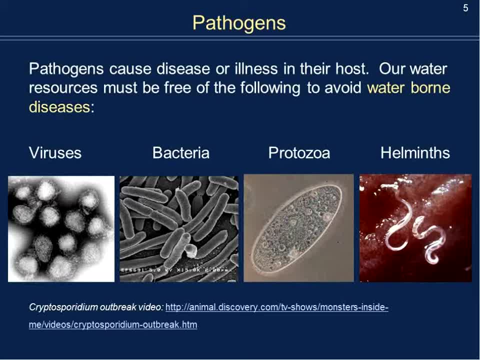 However, there are some bad organisms, And again, we say this bad in the sense that because they're called pathogens, And pathogens cause disease or illness in their host. Now, this depends on the type of organism. Not all microorganisms is harmful to humans. 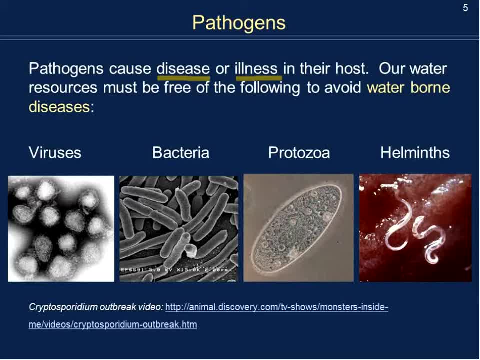 So it's just the ones that are concerned to us, so that if we ingest the hormone, not the pathogen, we are concerned about different types of diseases, The four that I asked you to consider. we're just going to talk about them and identify them now. 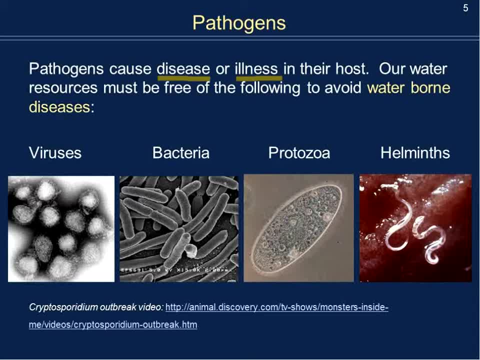 We'll talk about them in more detail when we talk about drinking water, When we talk about drinking water and wastewater, we'll point them out specifically. But again, we're going to be concerned about viruses, specific types of bacteria, specific types of protozoa and specific types of helminths. 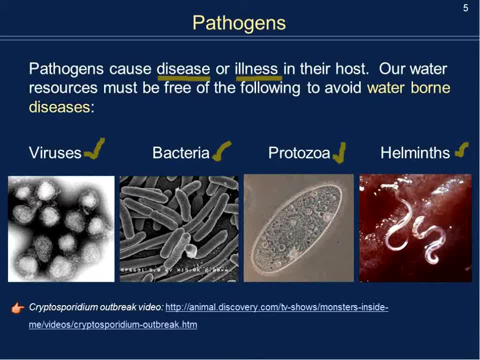 If you'd like- and again, this is a video I'll probably refer back to later on- cryptosporidium was a type of bacteria, if I remember correctly, And if you want to see a very quick video, This talks about how the outbreak of cryptosporidium affected many people in our country in the 1980s. 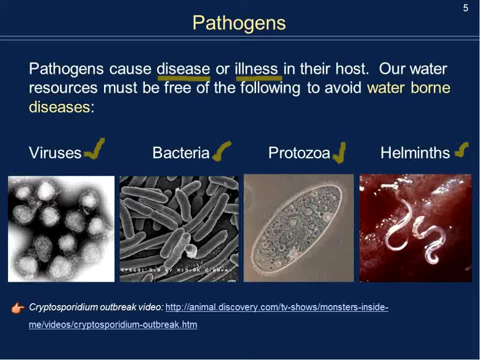 And it was once we learned that that we now will test to make sure that we don't have that in our water supply. Now we talked about the different types of microorganisms and pathogens. In order for organisms to survive, they have to break down organic materials. 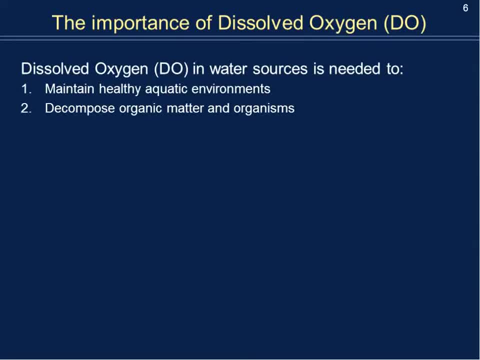 Again. think of it as food. They have to digest their food. In order to do that, you need dissolved oxygen. So what is the purpose of dissolved oxygen? You have to make sure you have enough in a water system so that you maintain a healthy aquatic environment. 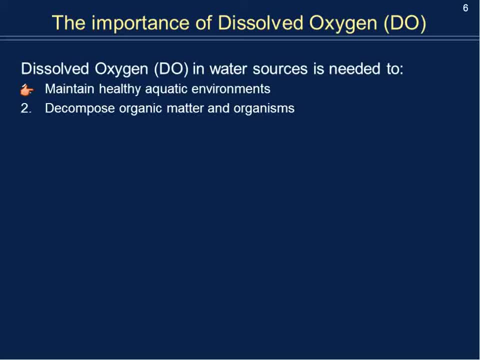 So, again, dissolved oxygen are like those- you almost want to consider them small oxygen bubbles, and many times they're microscopic. So you want to make sure that you have enough oxygen for the fish and other aquatic life to survive in the water. Also, you want to make sure that there's enough oxygen so that you can decompose organic matter, say in a wastewater system. 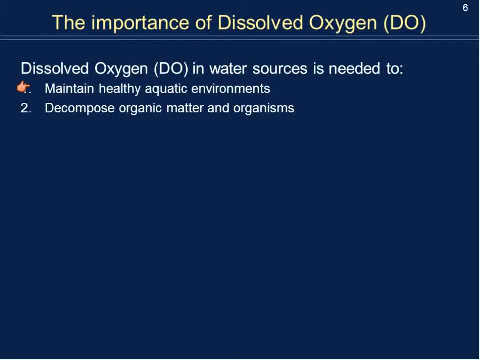 So again, these two are essentially the same purpose. The first: you want enough oxygen in a natural waterway. Second, you want enough dissolved oxygen in a treatment system. Now the question is how much? So we'll start talking about that eventually. 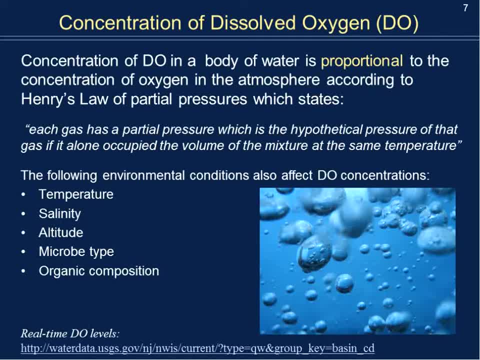 But the amount of dissolved oxygen depends on different types of systems, Different types of scenarios or different types of conditions. So you need to be concerned about temperature. You need to consider salinity, So again, the saltier the water source, again that will affect how much oxygen is needed to break down your organic matter. 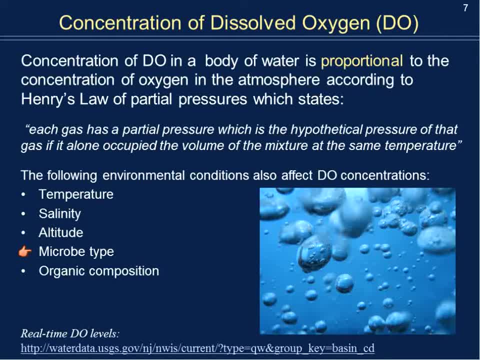 The altitude, The microbe type. So again, what organism is trying to break down the organic material And what is the nature of the organic material? We'll talk more about organic material in a moment, But again these are some of our concerns that you need to consider. 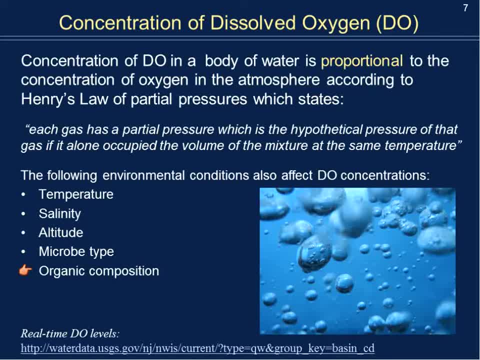 Now waterways are monitored constantly for the amount of dissolved oxygen that is present. If the water source is saturated with oxygen, that's the best scenario you can have, So 100% saturation is great. If there's very little oxygen present or those levels tend to go down, 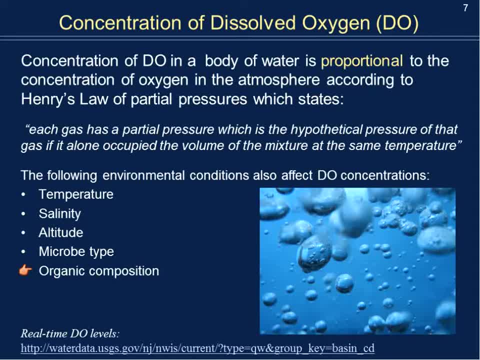 that means there's not enough oxygen for the marine life that's in the waterway. So I'd like to show you very briefly. This is an example of real-time water data from the United States Geological Survey. This is a government agency that has stations throughout the country at different waterways. 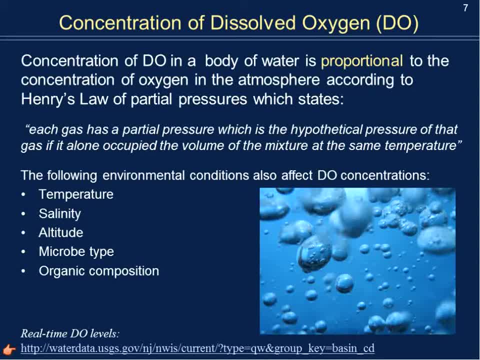 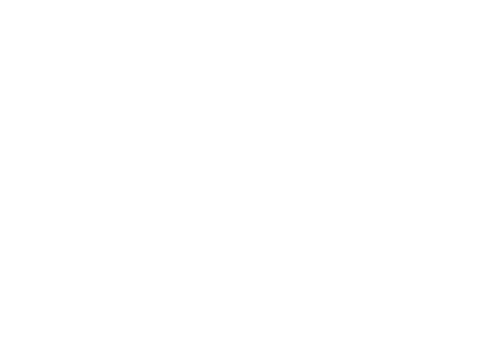 And they monitor the quality of our lakes and rivers. So I'm going to insert a new page here And I'll take an image from the website. Let's see, Give me just a second here to do that So you can bring that to you. 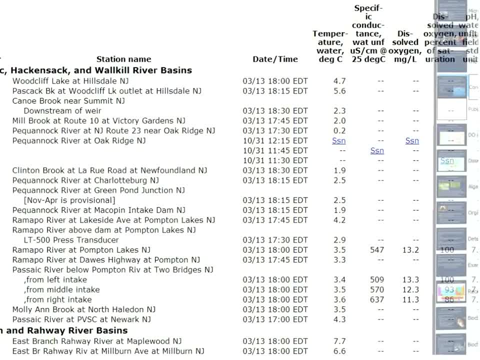 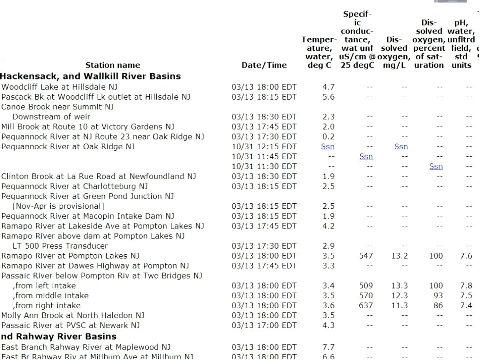 Unfortunately, some of my slides are shown there. Let's see if I can give you one more, better take on that. There we go. That's a little bit better to see. So this is actually from the USGS website And the one that I'd like to point out. there's some of the 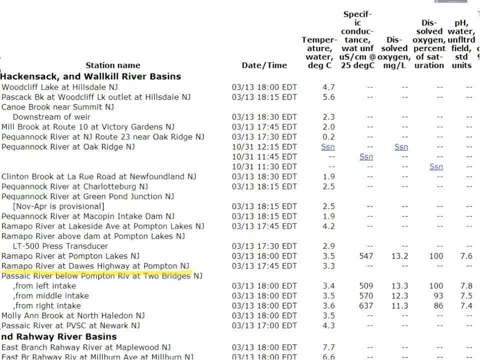 Here's some data from the Ramapo River at Dorse Highway in Pompton, New Jersey. Also the Passaic River below Pompton River at Two Bridges in New Jersey. If you look, this is the. If you look, this is the amount of dissolved oxygen in the waterway in milligrams per liter. 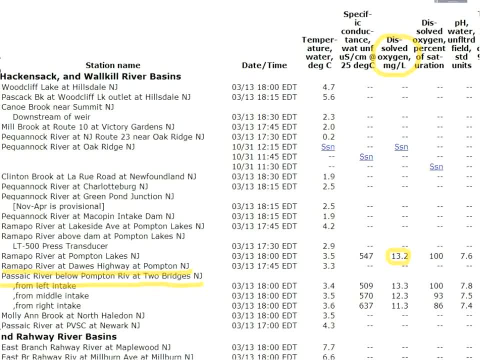 So in the Ramapo it's 13.2 at this time And in the Passaic River, at the station that's given, it's 13.3.. Why is that important? Again, these values are wonderful to see because if you look at the dissolved oxygen percent, saturation. 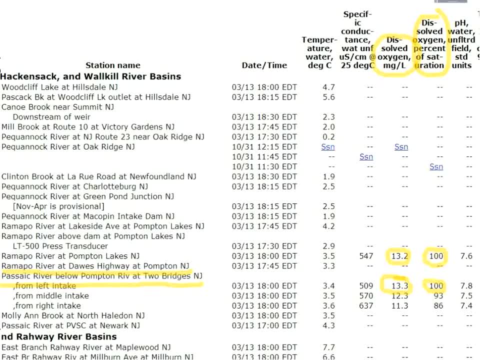 that means the waterway is 100 percent saturated. That means all of the oxygen that could possibly be in that waterway is available to the aquatic life. So this gives the impression that it's a very healthy system. If you notice that there's a section where it says the right intake, it's dropped quite a bit, about 86 percent. 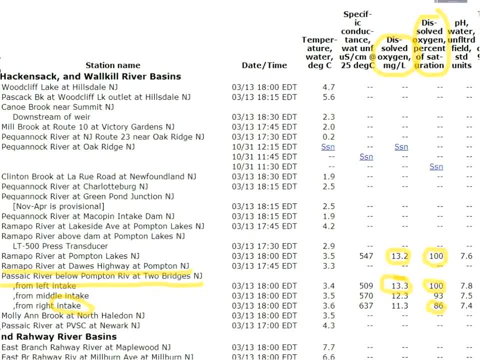 That means it might be more of a stagnant area with low velocity, And if that's the case, oftentimes fish will go there to hide or to find prey. So that might be an area where there's more activity and more oxygen. So again, that's something that they would monitor. 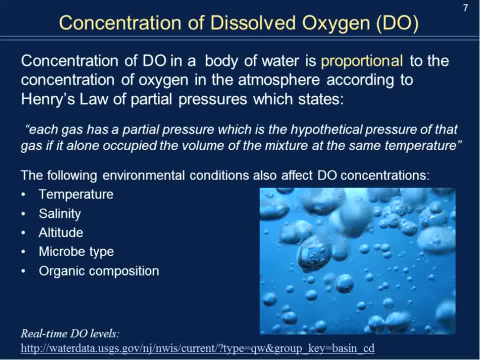 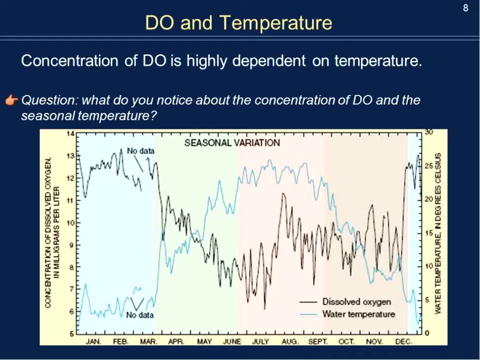 Now we talked also about again going back to some of our terms. we talked about temperature, So I'd like to show you a slide that talks about the relationship between dissolved oxygen and temperature. So the question I'm asking here: what do you notice about the concentration of dissolved oxygen and seasonal temperature? 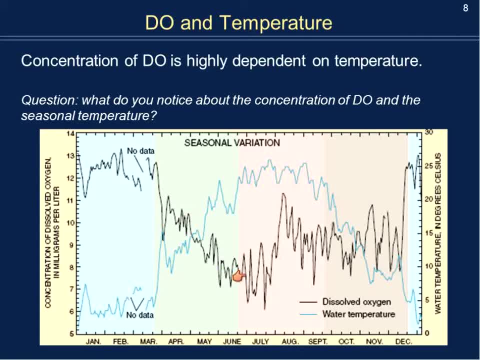 So if you notice the black one, that's the temperature, The blue one, that's the water temperature, And you can see that the blue line, as part of our scatter plot here, is the concentration of dissolved oxygen, while the blue shows the water temperature. 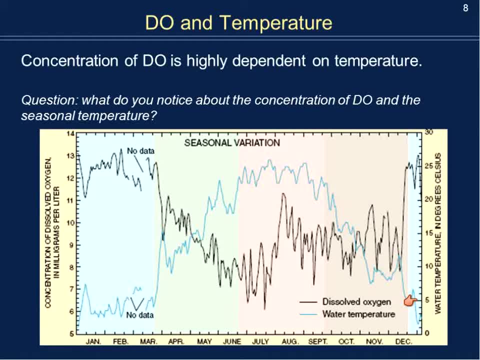 And you can see how it varies by season. Hopefully, you notice that there's an inverse relationship. Notice that the dissolved oxygen is high in the winter, when the water temperature is lower, While in the summer months the water temperature is higher but the dissolved oxygen is lower. 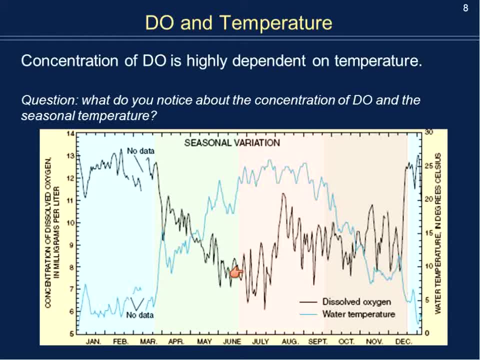 So the best way to describe that this all belongs to the partial pressure law, which essentially states that as temperature goes up, fluids move more towards a gaseous state and rise. So if you think about it- the best way you can think of this practically, if you've ever opened a soda or any type of carbonated beverage in the summer, you notice it goes flat a lot faster. 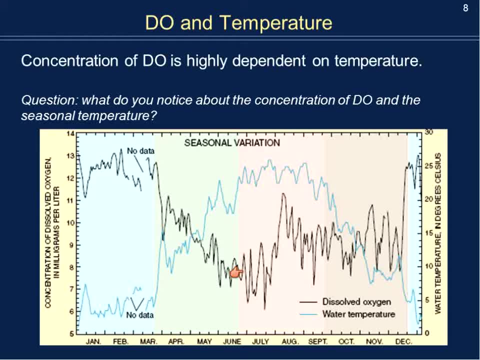 And the reason why is with the higher temperatures the gas bubbles readily move from the liquid into the atmosphere and rise So again, that's why your soda goes flat in the summer and not as quickly in the winter. And it has to do with the temperature to gas ratio, which in this case is the dissolved oxygen. 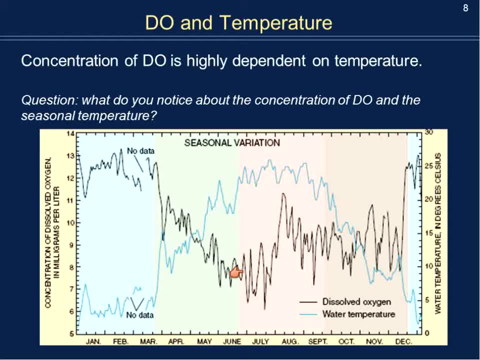 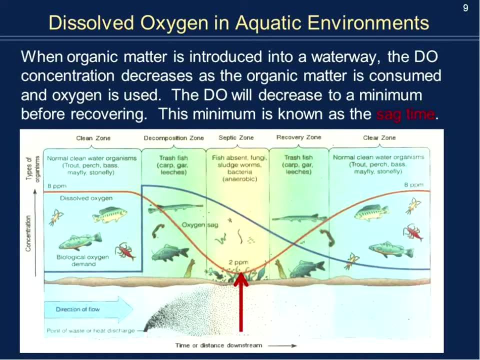 Dissolved oxygen also directly affects the aquatic environment, which we've mentioned before. But how? so Now say, a wastewater treatment plant is treating wastewater, so again, it's treating it in the plant and then suddenly releases it into an aquatic environment. 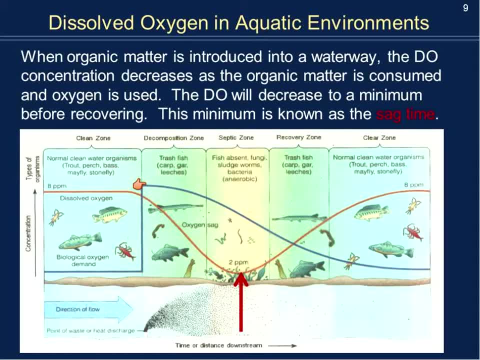 Well, when you release treated organic material, it's going to be broken down and oxygen is going to be used. Now, if too much oxygen is used in the system, that means there's no oxygen available for other aquatic organisms such as fish or lobsters or any type of aquatic plant life. 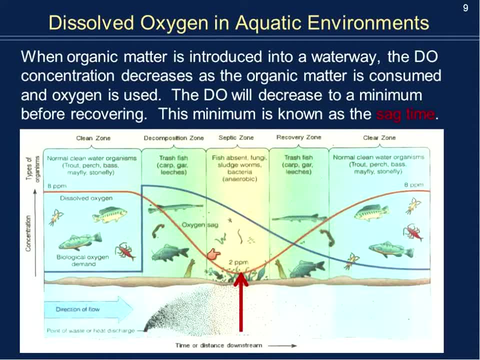 This point where you reach the critical two parts per million for dissolved oxygen is known as the sad time. So this is the amount of time it takes to reach the minimum amount of oxygen in a waterway. This is also part of what we call a septic zone. 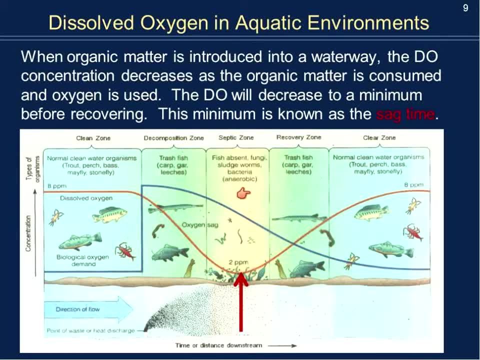 where only certain types of organisms can live in that type of environment, such as fungus, sludge, worms and bacteria, And this is because these types of organisms can survive on anaerobic respiration, meaning oxygen is absent. We'll talk a bit more about respiration and organic material in just a moment. 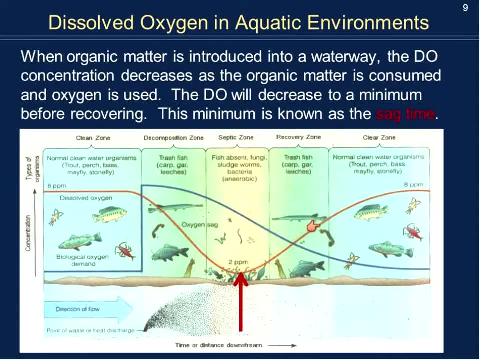 Now what happens is, as the system starts to recover and say fresh water moves into the system, say in a river, more oxygen comes into the system, which will allow the organic material to continue to be consumed. the organic material will reach a minimum. 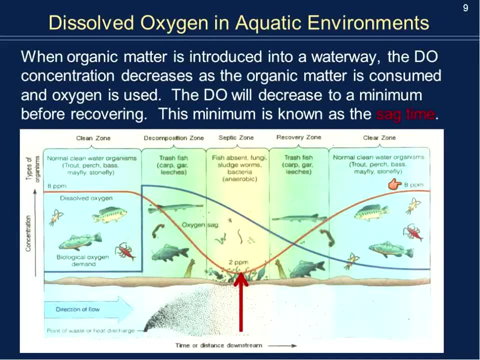 more fresh oxygen will come in, reach the healthy level of eight parts per million, and then you will see other aquatic life come back, such as trout, bass and other types of fish. So, again, it's really critical to have a healthy amount of dissolved oxygen in your waterway. 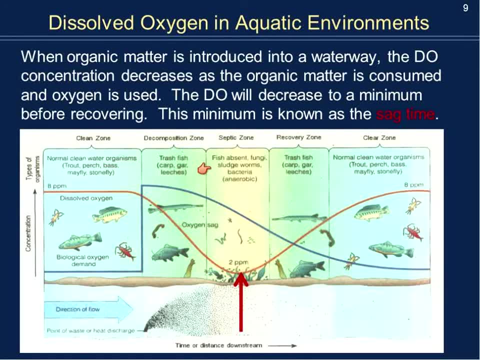 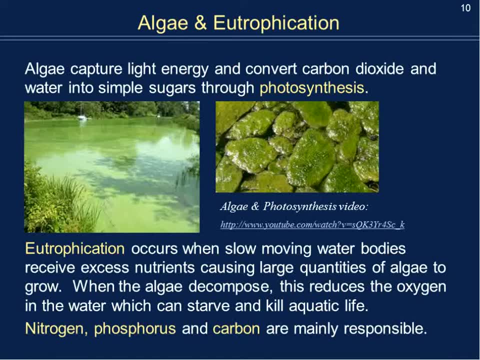 So what's an example of, say, a septic zone? What does a septic zone look like? Here's an example, And you've probably seen this before with certain waterways. This is also known as: one example of a septic system comes from eutrophication. 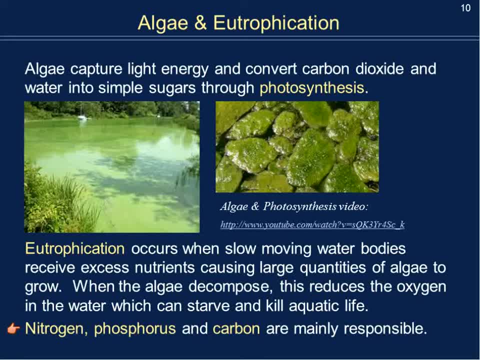 And what happens is when you put back into a system. so again say, if you treat water or maybe you have soil that has a large amount of nitrogen, phosphorus and carbon, what happens is that's an excellent food source for algae. 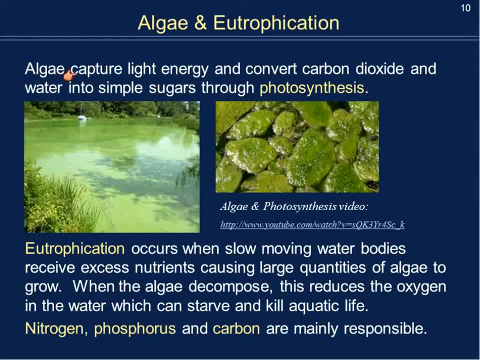 So algae use that as a food source, plus the organic matter coming in, and they convert both the organic material, the, not yet, excuse me. they convert the nitrogen, phosphorus and carbon and use light energy and convert that into carbon dioxide and water. 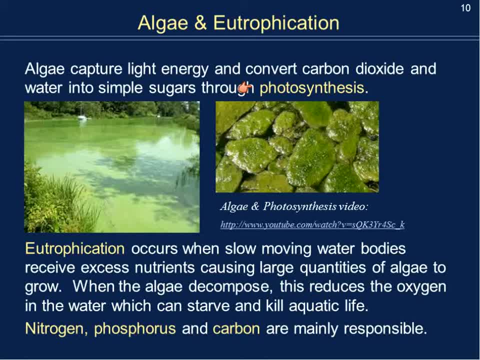 using the process of photosynthesis. That process of photosynthesis and the food source that the algae have causes them to reproduce and you get a system where that is just overflowing with algae. The algae consume all of the oxygen, and when you use all of the oxygen, 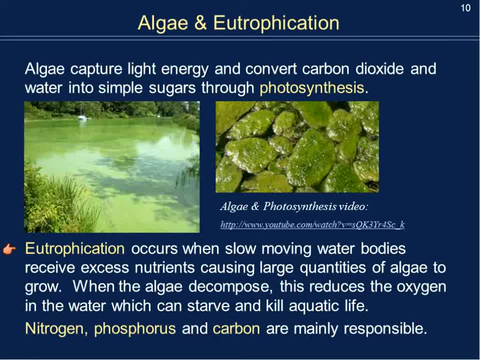 you get this eutrophication to occur Now. when that happens, essentially there's no oxygen left for any other organisms, so what you'll actually see is a large amount of aquatic life will die off because of that. So that's something we, as engineers, need to make sure. we 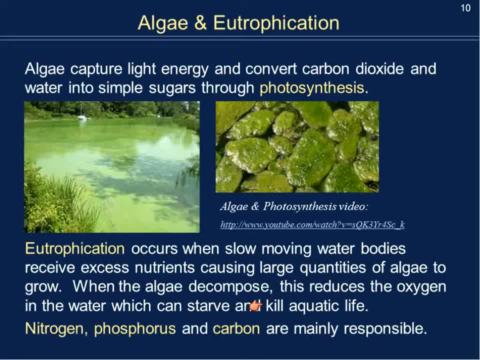 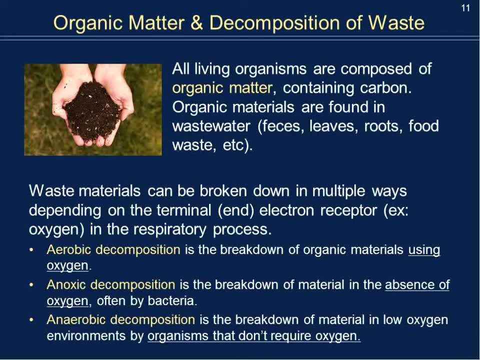 we monitor the health of a waterway to make sure there's enough oxygen for all of the aquatic life and not just the algae. Some terms we started to talk about, but we didn't define them as much. We didn't define what organic matter is considered. 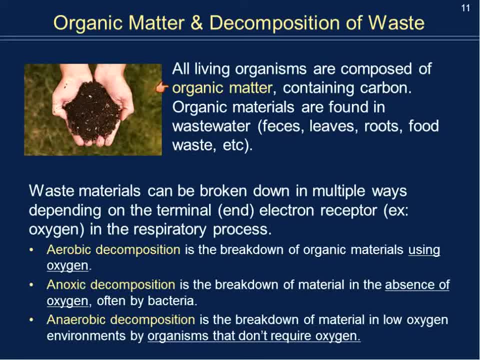 Organic matter is any sort of living organism or material that contains carbon. So again, the key term is carbon. Now, organic material can be found in our wastewater and drinking water in the form of feces, leaves, roots and food waste. 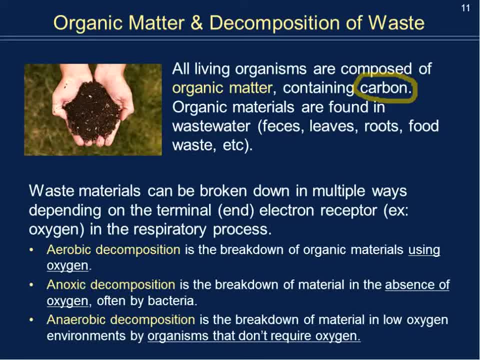 It's part of our job as engineers to remove that organic material so that we can have water that's safe to drink and safe to use. But how we remove it depends on three different types of methods, So we can often use good bacteria or good microorganisms. 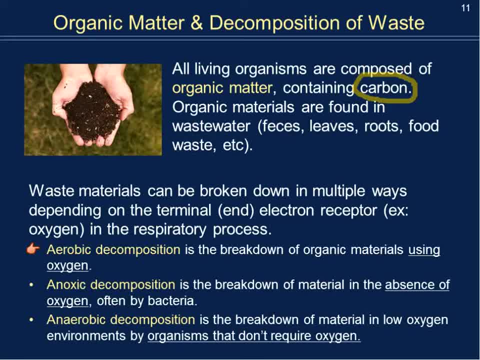 to break down the organic matter and remove it from the system so that we can purify our water. Our first method we could use is to add an aerobic decomposition, which has aerobic respiration, where the organisms break down the organic material using oxygen. That's very common. 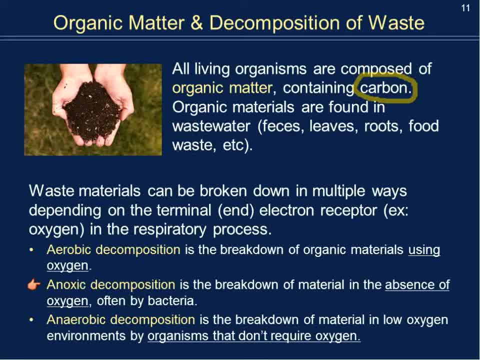 Or we can have an anoxic decomposition, where we have anoxic respiration by the microorganisms to break down material if oxygen is absent. Or you can have anaerobic decomposition, where you break down material with microorganisms when there's low oxygen and it's not necessary. 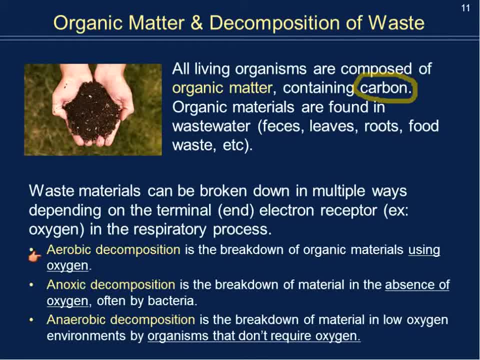 because the organisms don't require oxygen at all. So, again, depending on what type of system you have, you will look for a certain method of decomposition. Now, oftentimes one of our more popular ones is aerobic decomposition, using oxygen and breaking down materials that contain the carbon. 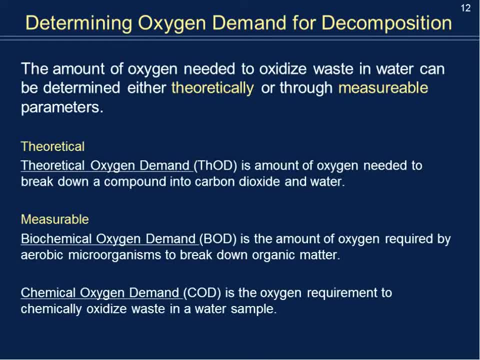 So how can you do that? How can you determine how much oxygen you need in order to properly break down organic material or to have a healthy aquatic environment? Well, the first method you can use is theoretical, in which case you calculate using the atomic weight. 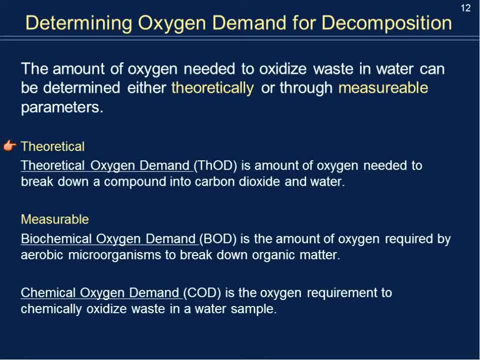 of the different organic substances, the amount of oxygen you need to break it down into carbon dioxide and water. Again, this is a theoretical method and, unfortunately, what's the downside of it is you aren't always able to account for all of the different variables. 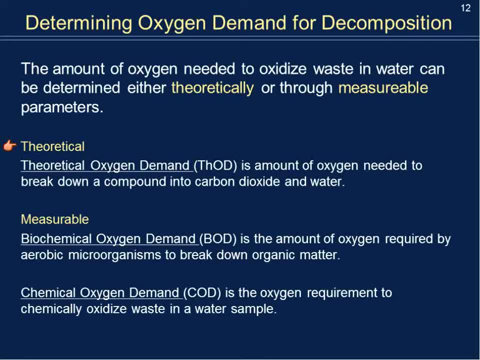 but usually you can get a very good value just as a starting point. Or you can use measurable means, which means you actually take samples of water that have organic material in it, put microorganisms into the sample and see how much oxygen they consume. 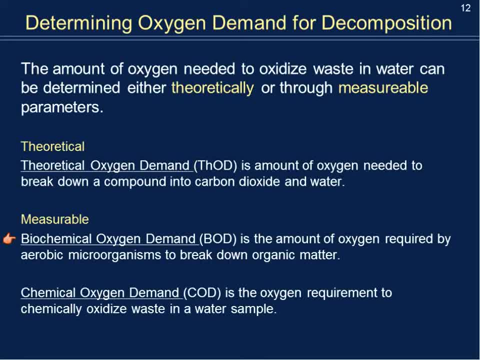 So, again, this is a very practical method. So you can either do that using biochemical, meaning using actual organisms as the method, or you can use chemicals, so you would have your organic material, you would add chemicals and then you would see how much oxygen in the water. 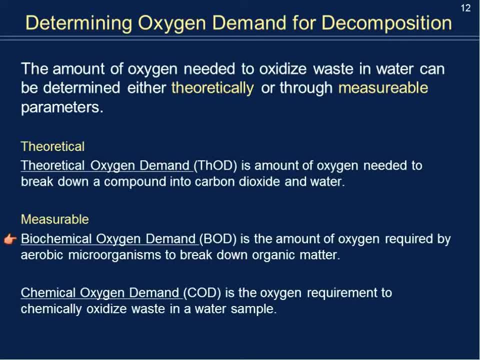 is used to break down that organic material. These are definitely the more common ways to go, simply because this is how we will break down material in a wastewater system. So what I'd like to do is my goal is to do one example of theoretical oxygen demand. 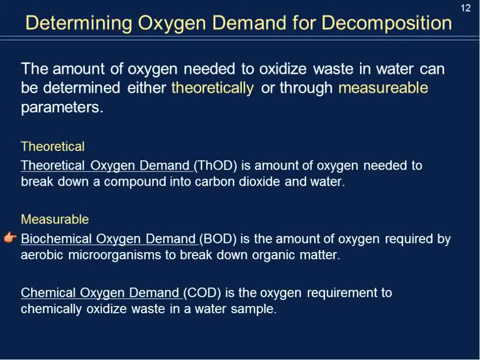 and an example of biochemical oxygen demand. Of the two, biochemical is very common because it's a natural system. So we'll do quite a bit on biochemical oxygen demand, or BOD. So example number one is the theoretical oxygen demand. 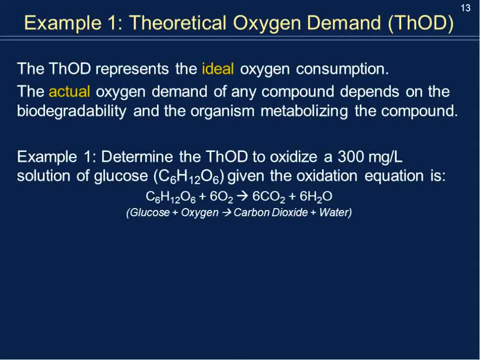 So theoretical oxygen demand represents the ideal oxygen consumption. Again, the actual amount of oxygen consumed depends on how easy it is to grade that substance or the organism that is doing, the metabolizer, which is actually consuming that substance. So oftentimes there's many different variables. 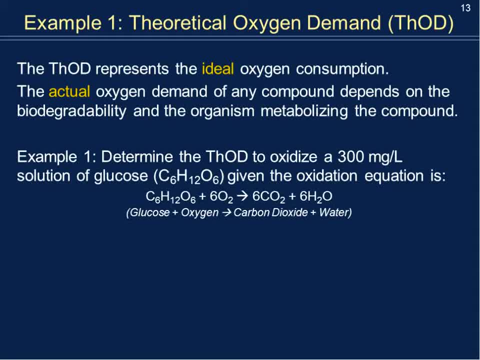 you need to consider but, like I said, it represents an ideal value and it gives you a starting point. What I'll be referring to- if you want to have up the PowerPoint and the video side-by-side- is I'll be referring to the periodic table of elements. 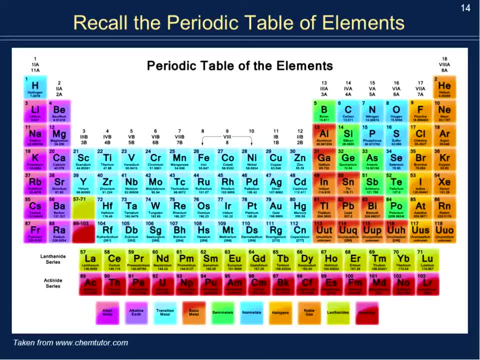 for atomic weight. That's the next slide on this video, So I'll be going back and forth to those But the three that you'll want to consider in particular, and I'll circle them for you just to find a color that works okay. 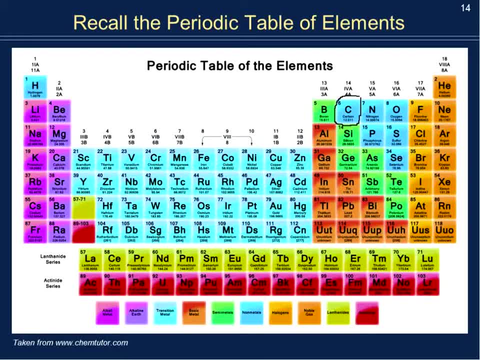 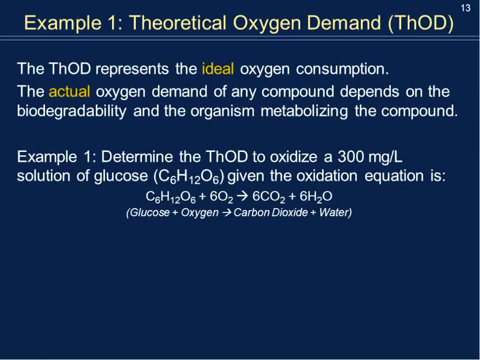 We'll be looking at carbon, oxygen and hydrogen, So we'll need the atomic weight of these three. So in order to solve the problem essentially, we're going to look at ratios: How much oxygen is needed in milligrams per liter? 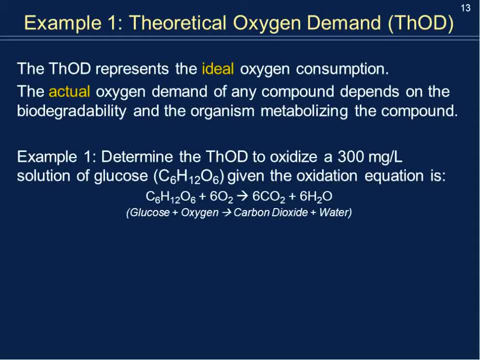 compared to how much glucose we're trying to break down. So here's an example. Example number one says: determine the theoretical oxygen demand needed to oxidize 300 milligrams per liter of glucose, which is C6H12O6.. 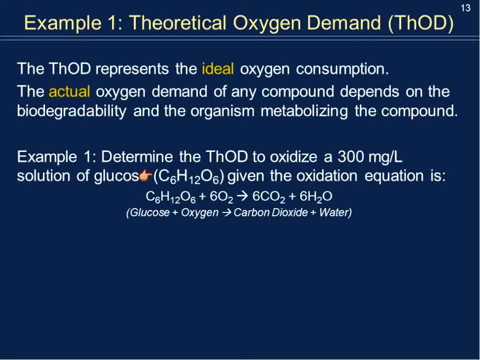 Probably many of you remember that from biology or chemistry. Given the oxidation equation is: glucose plus six double molecules or double bonded molecules of oxygen will yield six carbon dioxide molecules and six water molecules. So let's look at what the total concentrations of oxygen and glucose are. 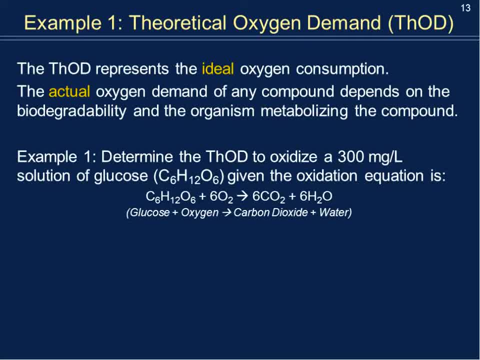 and let's see if we can work out a ratio. So first, let me start first with the glucose. So first we're going to determine, let's say, atomic weight, That's, so we can determine their concentrations. So first with the glucose. 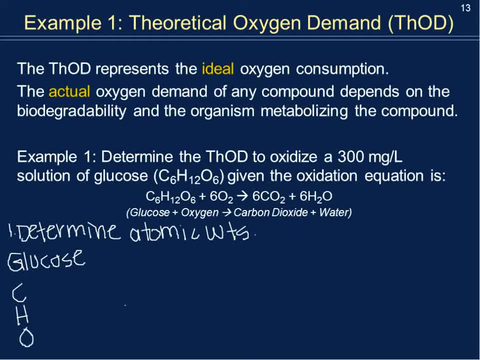 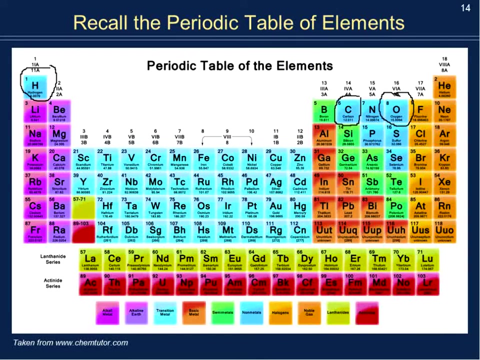 we have carbon, hydrogen and oxygen. The carbon has six molecules, the hydrogen has 12 molecules and the oxygen has six. So we want to multiply that by their atomic weight. So let's look real quick, Going to our periodic table. 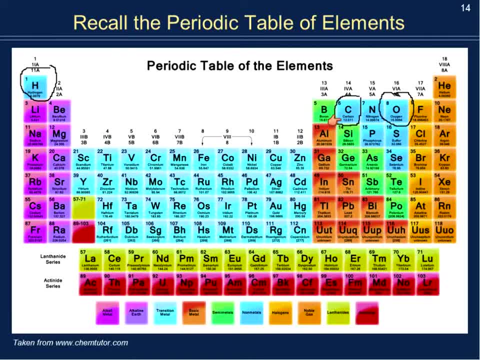 carbon- and I do apologize, it's very hard to see. You might want to zoom in, if need be. Carbon has an atomic weight of approximately 12.. Oxygen has an atomic weight of approximately 16.. And hydrogen has an approximate atomic weight of one. 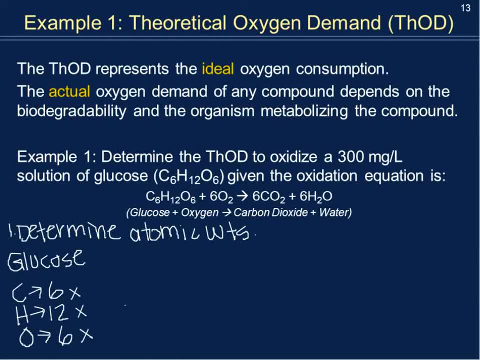 We'll use that information in our problem. So again, we said carbon has an atomic weight of 12.. Grab my pen here. Hydrogen has an atomic weight of one And oxygen has an atomic weight of 16.. So let's find out what the total atomic weight is. 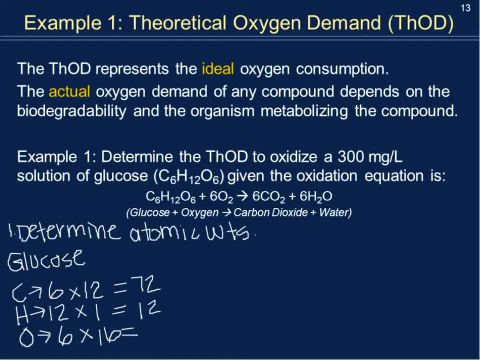 So we have 72,, 12, and 96. That gives us a total of 180 to the atomic mass. Now let's do that for the oxygen as well, so we can see what the ratio needed is. We know we have 300 milligrams. 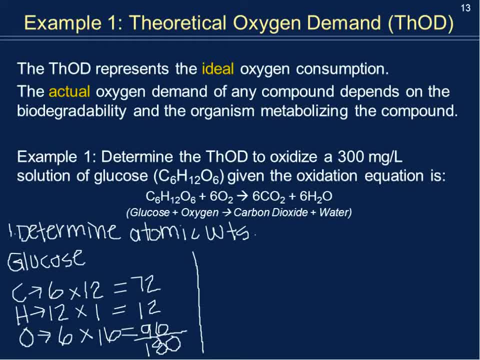 per liter of glucose. So again, we want to see how much would we need to oxidize the oxygen So we have for our oxygen? we're working only with oxygen molecules, of which there are 12, because, again, just to point out, 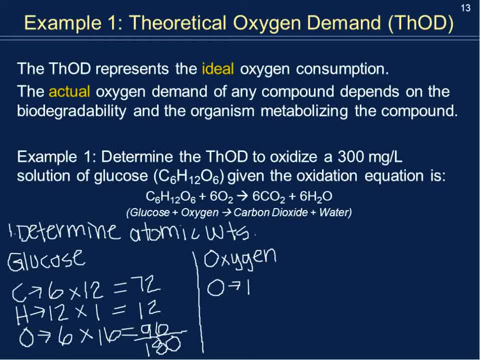 you have six double bonds, So that's a total of 12 molecules, And oxygen has an atomic weight of 16.. That gives us 192.. So notice: the glucose has an atomic weight of 180.. Oxygen has an atomic weight of 192. 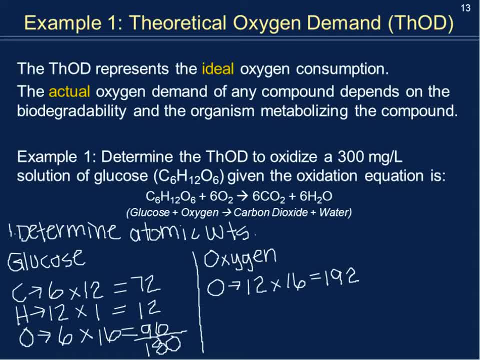 So it's actually more So. now that we've determined the atomic weight for step two, let's determine concentration of the oxygen needed. We'll talk about that in a little bit. Looks like I'm a little delayed with my writing here. 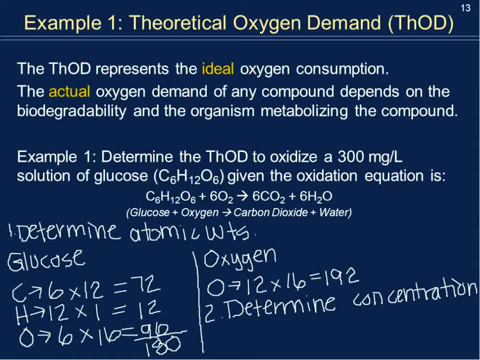 Concentration. there we are. So what's the ratio? The ratio of oxygen to glucose, And we want to multiply that by the concentration of- and again, this is just a simple ratio- times the ratio of glucose, which is 300 milligrams per liter. 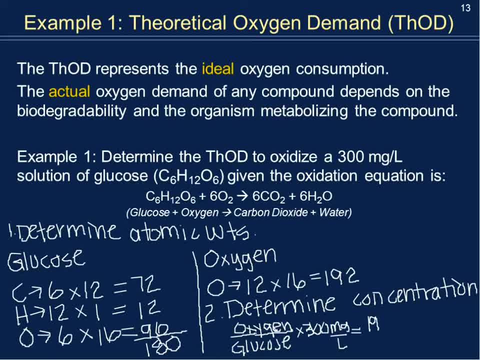 So if that's the case, we have oxygen with an atomic number of 192, glucose with an atomic number of 180, times a concentration of 300 milligrams per liter. Again, all this originally was was a ratio of atomic number oxygen to glucose equals. 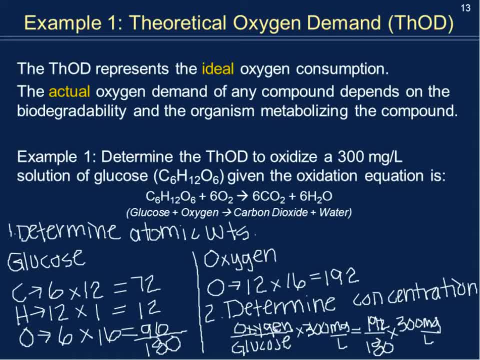 oxygen to glucose. So we did atomic number to atomic number, concentration to concentration And my numbers are a little bit squished, but hopefully you get a concentration of 321 milligrams per liter. So you need 321 milligrams for every liter of water of oxygen in order to break down. 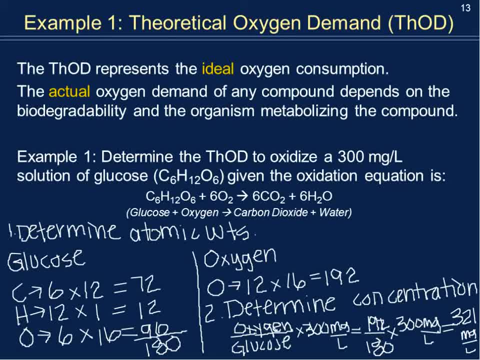 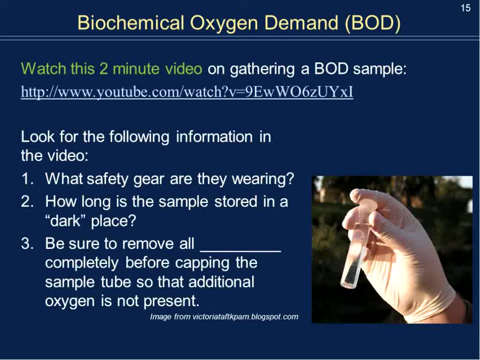 the glucose and oxidize it into carbon dioxide and water. So, again, that would be the theoretical oxygen demand. Now we've talked about the theoretical, let's talk a little bit about the measurable means, Again, the first being the biochemical. What it asks you to do, and, again, just to do this, it's a quick two-minute video. it 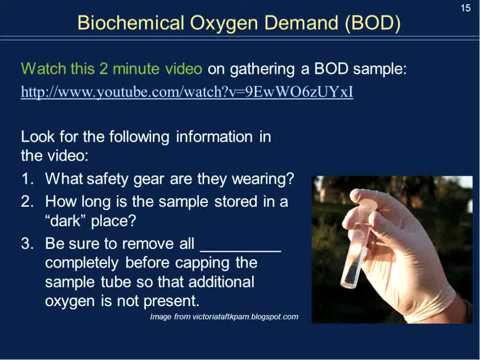 talks about how you would gather a sample to measure biochemical oxygen demand. So take a moment, pause the video, but make sure you think what the answer is for these three questions. What safety gear are they wearing? How long is the sample stored in a dark place? 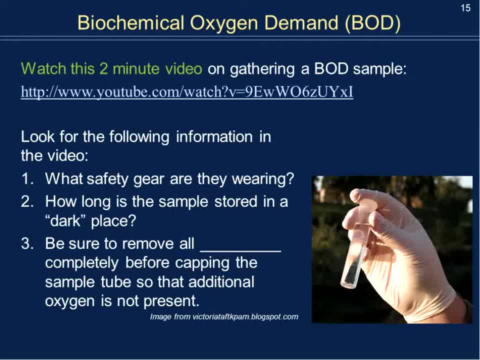 Be sure to remove all of what completely Before capping the sample tube, so that the additional oxygen is not present. So I'll give you a moment to pause and then we'll resume. Now, after watching the video, you want to focus on the fact that they're wearing safety. 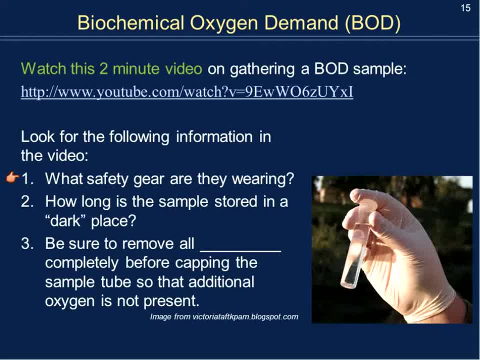 gear, particularly because if you're collecting a sample, your sample may have pathogens in it. And again, you don't know what types of microorganisms. Okay, You don't know what types of microorganisms you have. Some are good, some are bad. 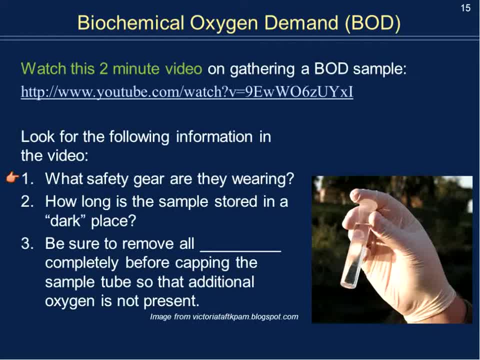 So you just want to make sure that you're protected. Second, you want to make sure you store the sample for five days in a dark place, And we'll explain why. And finally, when you cap your sample- and the one that's shown here is actually not- 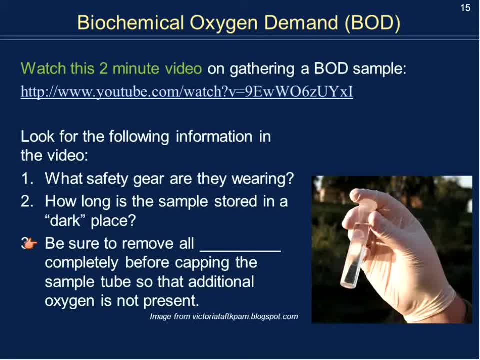 a good sample, because there should be no air present. You want to make sure you remove all the air so that you don't introduce additional photosynthesis Again. photosynthesis requires oxygen, Additional oxygen. oh, I'm sorry, let me rephrase that. 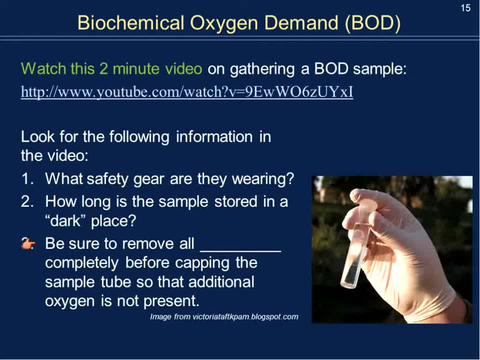 You put it in a dark place so that you don't have photosynthesis, but you want to remove additional oxygen that might be present in air, so you fill the entire sample so that you don't have air contaminating part of your test. So this is a brief rundown of how you would measure the amount of oxygen needed using. 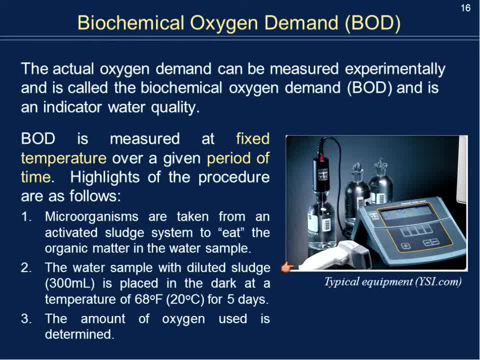 biological systems. So again, the system essentially looks like this. These are your samples that you've collected water, so again, you typically make sure you fill it to overflowing. These are approximately 300 milliliter samples. This is the typical volume that's used. 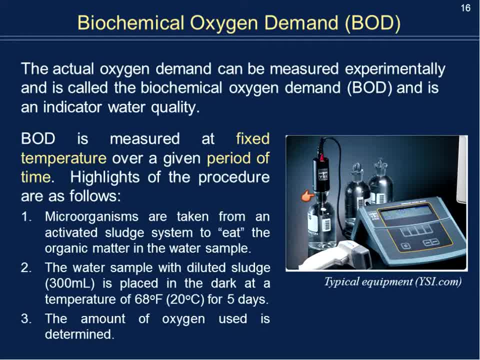 And then the five-day value which we will get to is what you're measuring. So how do you measure the BOD over the five days? Well, first you measure the BOD, You need a source of organisms, organisms that will break down the organic matter. 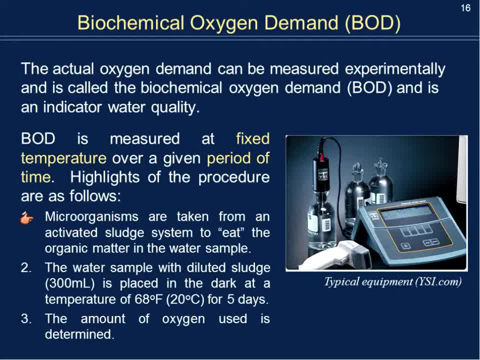 The organisms can either be taken from, say, a waterway- so again if you're testing to see if there are any organisms present- or you can take it from what we call an activated sludge system, which essentially means you remove good bacteria from a wastewater system. 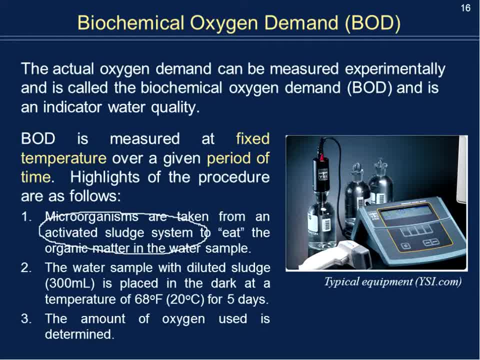 So what you're doing is you're removing good bacteria from a wastewater system and you're removing good bacteria from a wastewater treatment system, And what that does is that provides the organisms to eat the organic material. So then you get a water sample which has organic material in it. 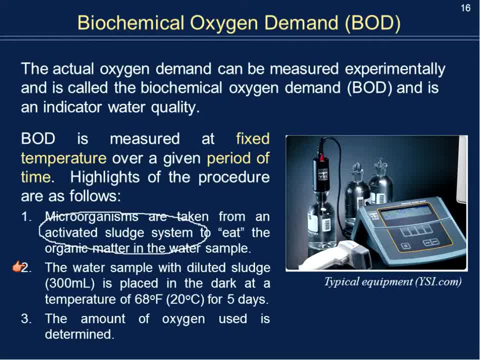 You place it in a dark location for five days at a constant temperature of 68 degrees Fahrenheit, with the microorganisms added in so that they can consume the BOD, And in the process they also use oxygen. At the end of the five days you measure how much oxygen remains. 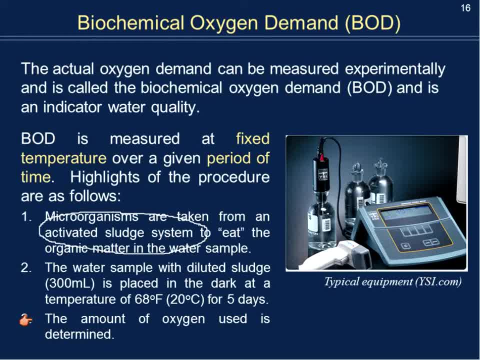 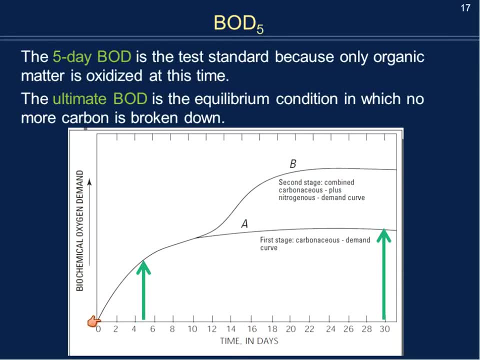 So again, first you test to find out how much oxygen is present before you take the test, and then you see how much oxygen remains And that tells you how much oxygen was used, The reason why we use five days, which we call the BOD-5, so if you were to plot the 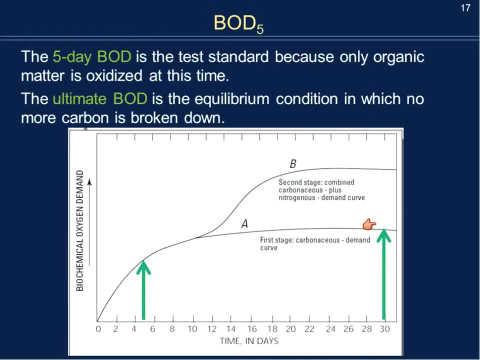 amount of oxygen used over time. you would see that it's an exponential curve and it's a negative exponential curve. The reason why the test is for 5 days is it gives you a good sense of the amount of oxygen that's needed over a short period of time, And this is what 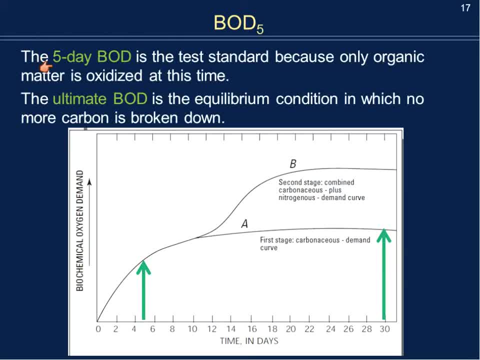 we call the BOD-5, or the 5-day BOD, And one of the reasons we use this is that the 5-day BOD is when only organic matter is oxidized at that time, Where the ultimate BOD, if we 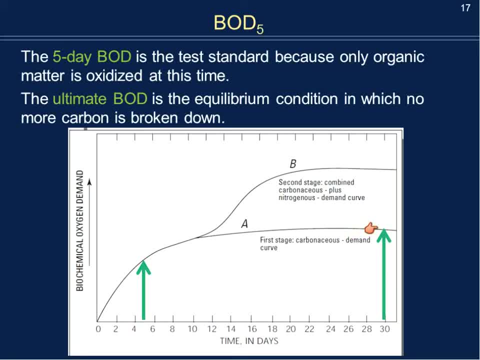 follow. the curve is essentially where the curve reaches equilibrium. so again, it starts to plateau And this is where no more carbon is broken down. this is an equilibrium position. This secondary curve also contains a nitrogen breakdown. So again, we're not considering that. we're only concerned about curve A, which is an 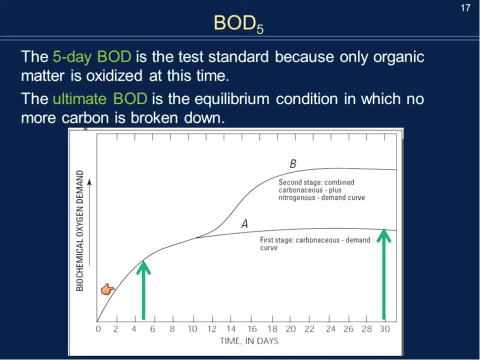 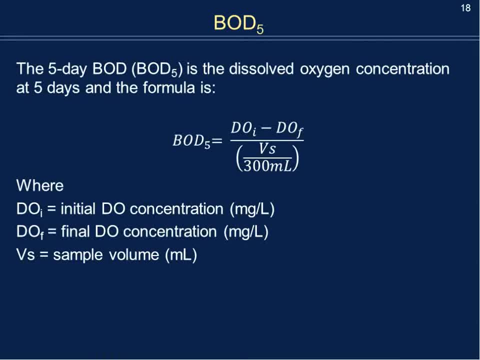 exponential curve and it's only of carbon breaking down. So how would you determine the BOD concentration for 5 days? Again, it's essentially a ratio. Again, you look at what was the initial oxygen concentration when you started, what was the 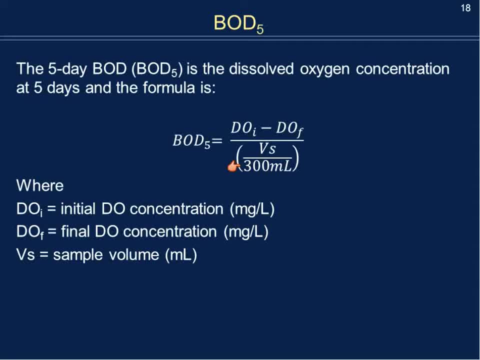 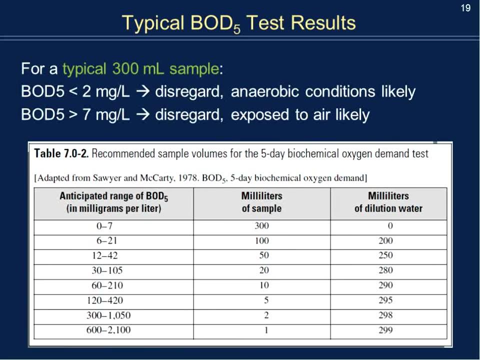 final oxygen concentration after 5 days And the test is standardized based on the number of 300 milliliter samples. So what you do is you take a ratio of the volume of your sample that you used and compare it to 300 milliliters. Typical test results, assuming 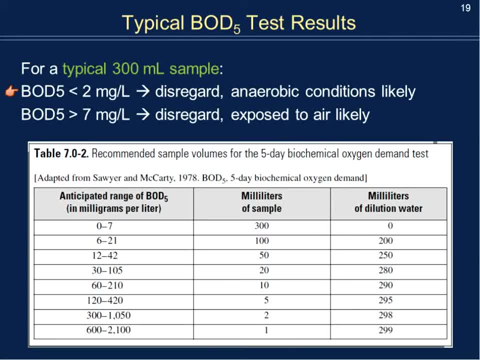 you have a 300 milliliter sample. if the BOD-5 is less than 2 milligrams per liter, typically you get rid of it, And the reason why that means that there's a very small amount of oxygen present and most likely anaerobic. 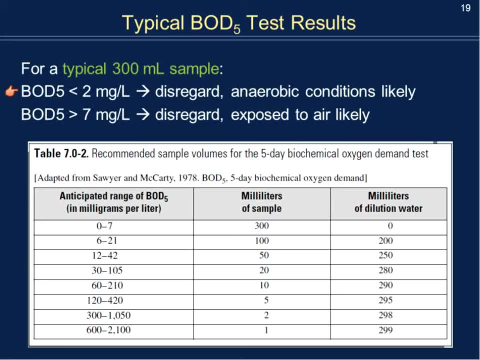 And the total CO2 that's released from the BOD-5,- that's the carbohydrate, And it's very difficult to determine if there's any decomposition or anaerobic respiration occurring, which means the test is not even valid because the material is being broken down by organisms. 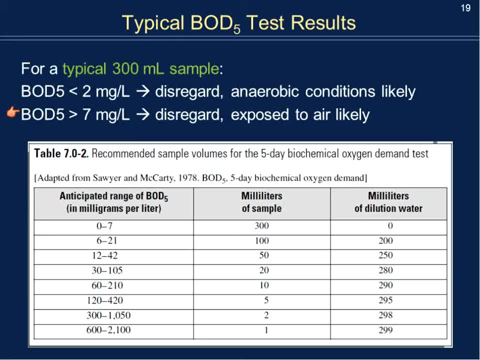 that don't even need oxygen, So it's a test that's invalid. Now, if it turns out that the BOD-5 is greater than 7 milligrams per liter for a 300 milliliter sample, we still disregard it, typically because most likely air got into the sample. And if 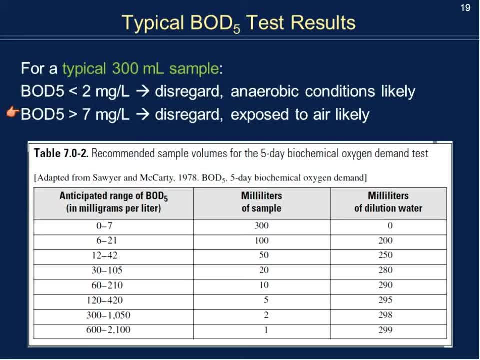 highly concentrated with oxygen, it's a false reading. So again, for a 300 milliliter sample, you don't need to dilute it because that's the standard value and typically you'll see a range of 0 to 7, but, like we said, we typically disregard values below 2 and above 7.. And 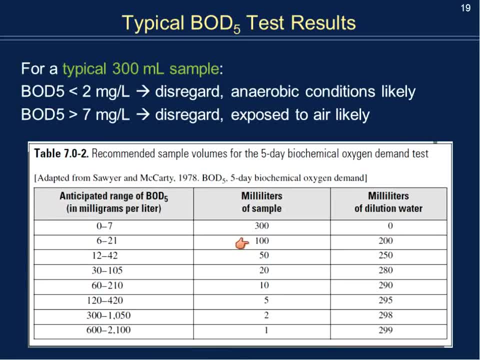 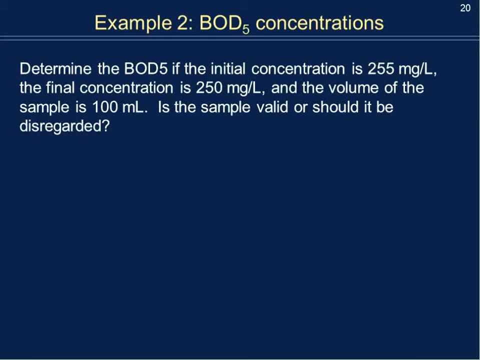 if you want to scale your test based on the amount of sample present. these are the anticipations for the BOD in milligrams per liter. So if that's the case, let's try to calculate a BOD concentration. So the question says: determine the BOD5 if the initial concentration is 250,. 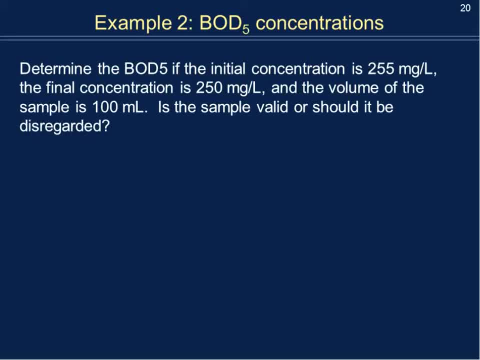 255 milligrams per liter and the final concentration is 250 milligrams per liter, And the volume of the sample is 100 milliliters. Now, keep in mind 100 milliliters is less than the standard value would need to scale it. is the sample valid or should it be disregarded? So for step number, 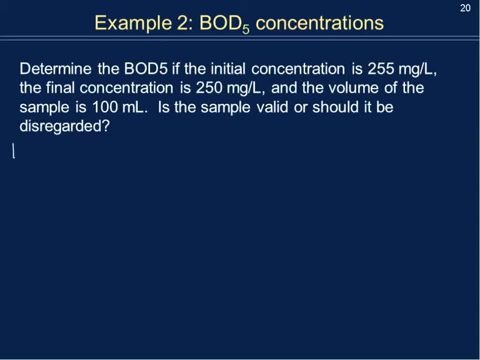 1,. first let's determine the BOD5.. So again, the BOD5 is equal to the initial concentration, which is 255 milligrams per liter, minus the final concentration, which is 250 milligrams per liter, and we have to scale our ratio based on the 100 milliliters that we have. 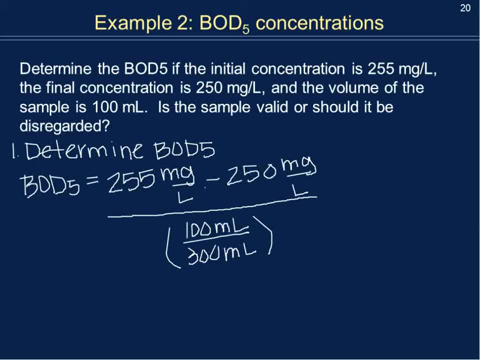 compared to the 300 milliliters of the standard sample. Take a moment, try to calculate it. If you need to pause, please do. Hopefully you got a concentration of 15 milligrams per liter. Is that valid? So for question. 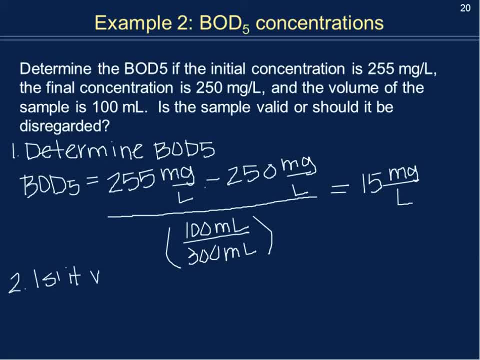 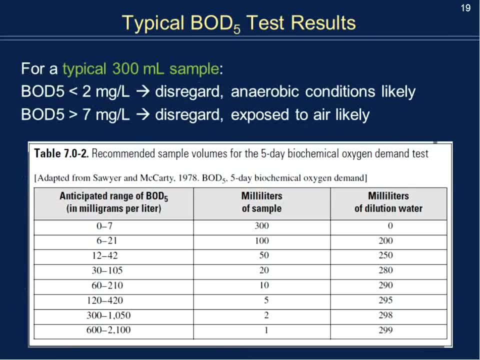 number 2, is it valid? Well, let's see If we go back to our table. just before I'll grab my highlighter. our sample was a 100 milliliter sample and the anticipated range should be between 6 and 21.. So in that sense, yes, we'll say that it is a valid sample. 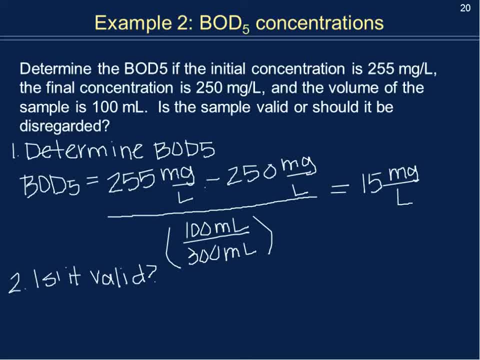 Sorry, going back to my problem here. So is it valid? Yes, because 6 milliliters- or 6 milligrams per liter, excuse me- is less than or equal to 15 milligrams per liter. So that's correct. So we have 21 milligrams per liter. So now that we have that, let's move on and 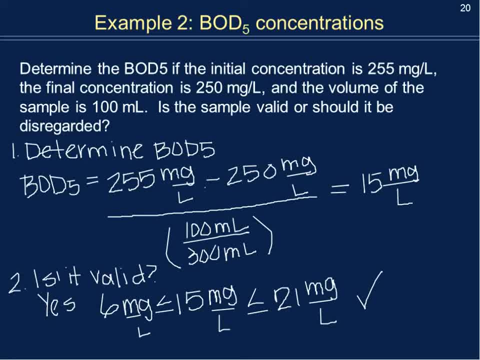 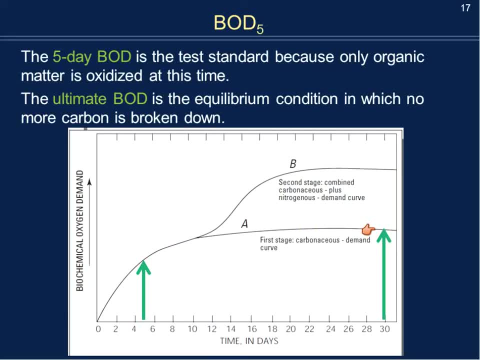 talk about another term, which is the ultimate BOD, And again, we talked about that just for a moment when we said that when the amount of oxygen starts to reach an equilibrium, meaning no more oxygen is being used or no more carbon is being broken down, this is 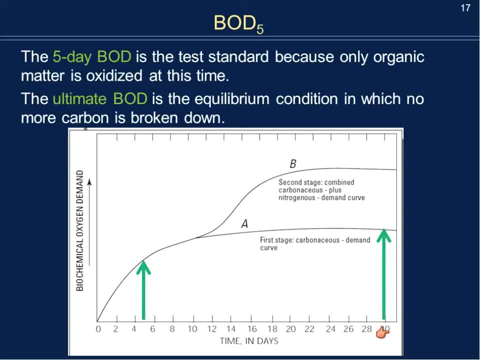 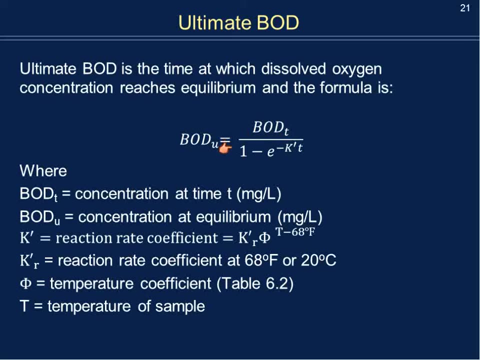 known as the ultimate value. so it's essentially at what time, meaning in how many? typically, how many days does it take to reach that ultimate concentration or ultimate oxygen demand? So the ultimate BOD is again an exponential equation. so notice, it's a negative exponential. 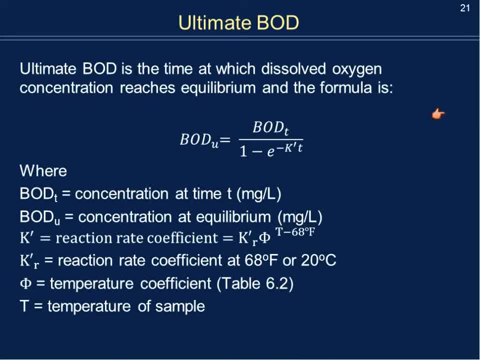 because we have a plateau as opposed to a positive exponential which ramps up. What do each of the terms stand for? The BODT stands for the BOD at any specific time. Usually we start with the five-day value that we've tested and gotten the concentration. 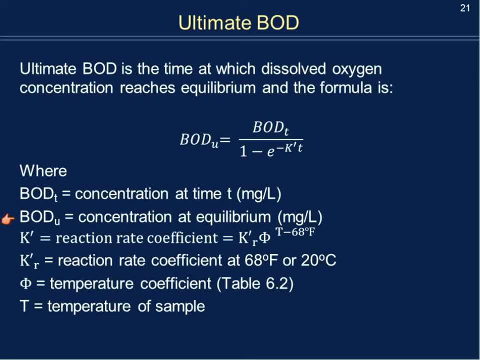 for so that we can find some of our other values. Again, the ultimate BOD is the value of equilibrium, so that we can project out at what time will we reach our equilibrium position. K prime is the reaction rate coefficient and again this depends on multiple different. 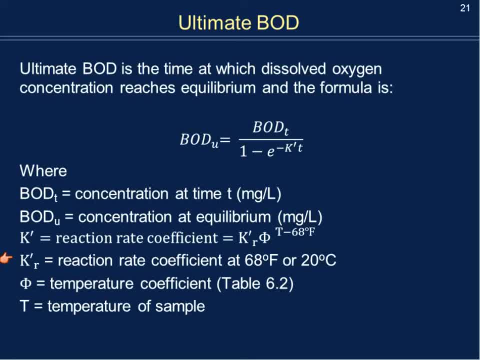 variables. Often this is determined in the laboratory. K prime sub R is the reaction rate coefficient at 68 degrees Fahrenheit or 20 degrees Celsius with standard value, which is what we'll use in the next problem. There's a temperature coefficient if you shift from the standard range of 68 Fahrenheit or 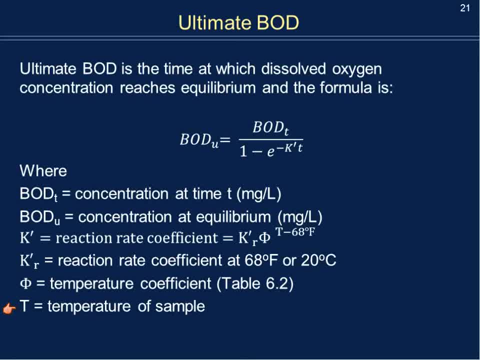 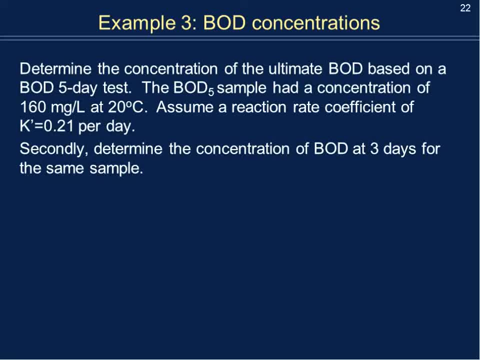 20 Celsius and then the actual temperature, for example. So again, let's try example number three, which is again a BOD concentration. It says: determine the concentration of the ultimate BOD based on a BOD five-day test. The BOD five sample had a concentration of 160 milligrams per liter at 20 degrees Celsius. 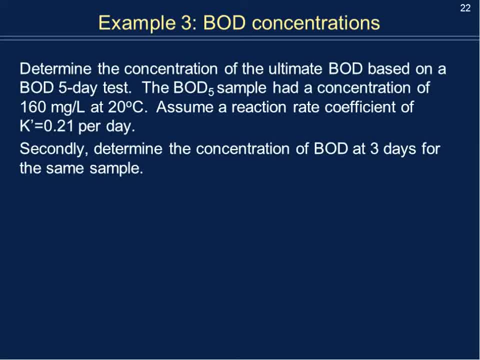 That's good to know, because that's the standard temperature, so you don't have to alter your K prime value. It says: assume a reaction rate coefficient of K prime equal to 0.21 per day. So again, since the K prime value is tested at 20 degrees Celsius, we're going to use 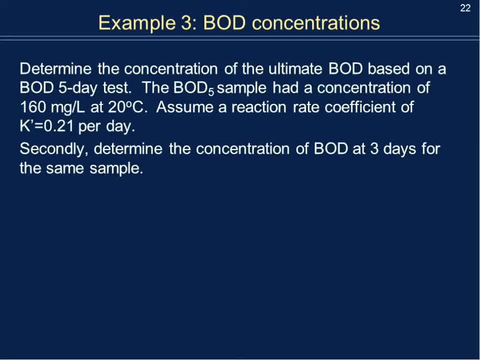 the BOD five-day test to determine the concentration of the ultimate BOD at 20 degrees Celsius. You don't have to alter it. Secondly, we're asked to determine the concentration of biochemical oxygen demand at three days for the same sample. So let's do step number one. 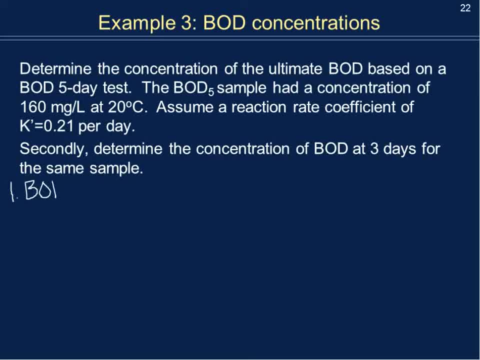 So first we are asked to determine the BOD ultimate, And I'm going to go right into the equation. So the BOD ultimate, The BOD ultimate is equal to the BOD five concentration, which is 160 milligrams per liter, divided by the exponential equation, which is 1 minus E, to the negative K, which. 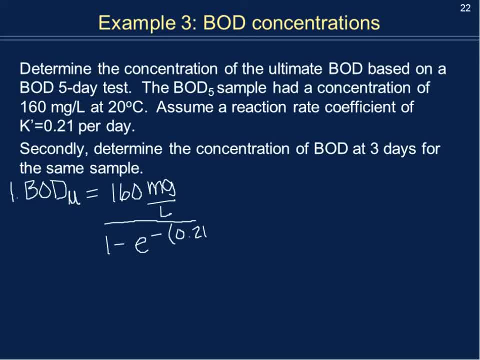 is 0.21 per day multiplied by five days, Because that's the BOD five-day test. Okay, Now, if you do your calculations, you're going to get a value of 246 milligrams per liter. So that's the concentration of oxygen used. so that's the oxygen required after five days. 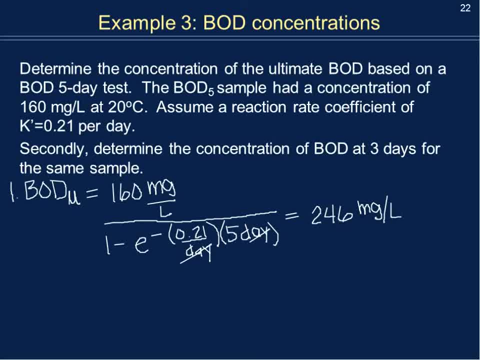 Now, excuse me, no, not after five days, excuse me. That's the amount of oxygen used, So that's the amount of oxygen required. That's the amount of oxygen required at equilibrium, the ultimate value, So O2 needed for equilibrium. 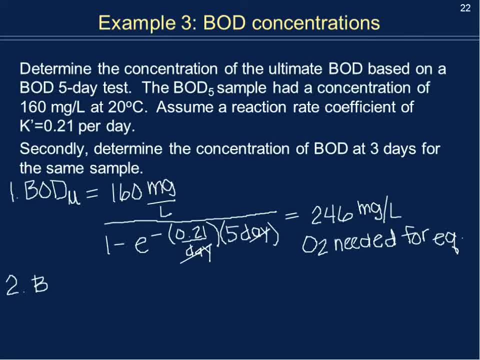 Now, using that information, let's calculate the BOD3.. Now notice, with our equation here, the BOD ultimate is a standard- or I shouldn't say standard, but constant value, and it's more an equilibrium value. What typically will change is the BOD at a certain time, and again that time is listed. 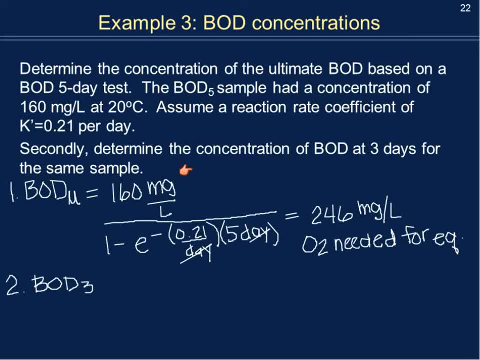 here. So what I'm going to do is I'm going to solve for BOD at 3 days, so my equation gets rearranged such that the BOD3 is equal to the BOD ultimate. Okay, Multiply by 1 minus E to the minus K prime T, So solving for BOD3, again we just found: 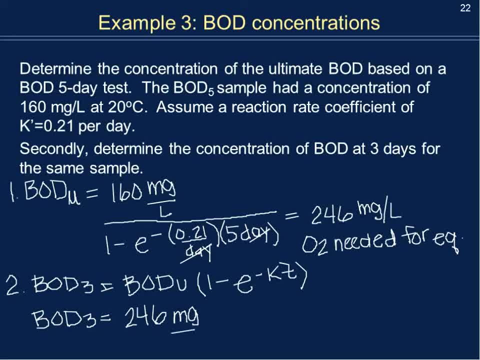 our ultimate BOD to be 246 milligrams per liter. Multiply that by 1 times E to the 0.21 day. Now times 3 days and our days and days cancel. If you calculate that, you should get approximately 115 milligrams per liter. 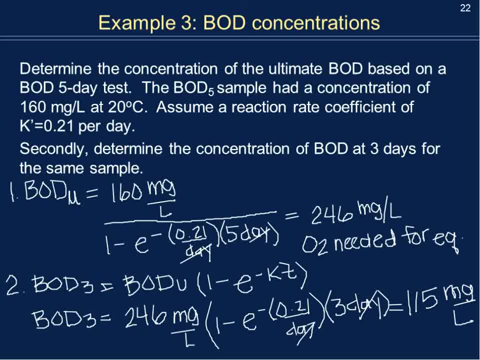 So that's how much oxygen is needed at day 3.. So now, if you notice, we've spoken about the theoretical oxygen demand. We've now done one of the measurable types of oxygen demand calculations, which is the biochemical oxygen demand. Our last type of oxygen demand is chemical oxygen demand. 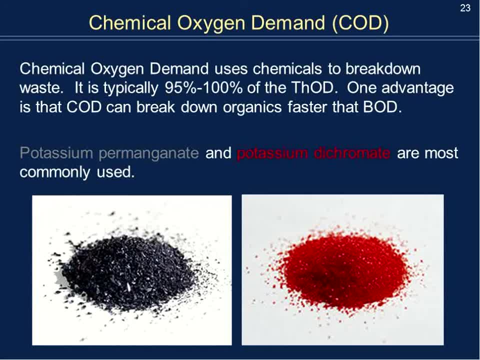 So, again, this is a measurable method to determine the amount of oxygen needed to break down organic material. So chemical oxygen demand, instead of using organisms, uses chemicals to break down the amount of oxygen. So, again, the highlight is that we're using chemicals instead of organisms to break down. 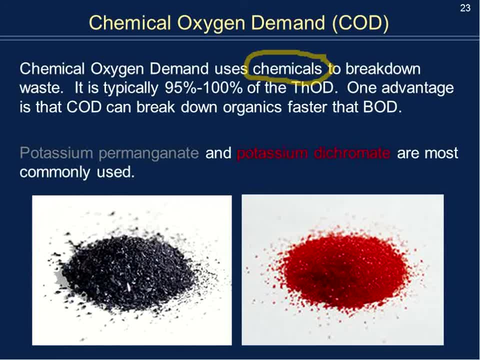 waste or organic material. What is ideal is: typically the chemical oxygen demand turns out to be 95 to 100 percent of the theoretical oxygen demand, So it's a very efficient way to break down waste Also. another benefit is that the chemical oxygen demand turns out to be 95 to 100 percent. 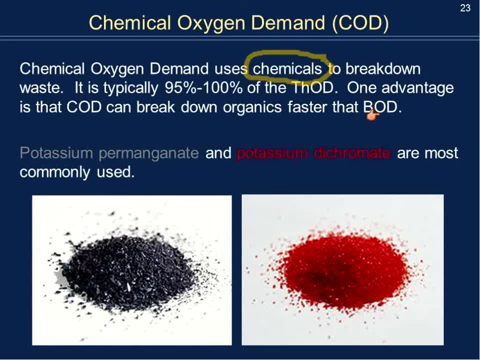 of the theoretical oxygen demand. So that means that the chemical oxygen demand can break down organics even faster than the biological oxygen demand. So the question would say: why would you choose even to use the biochemical oxygen demand? Well, the reason why is because it's a natural system. 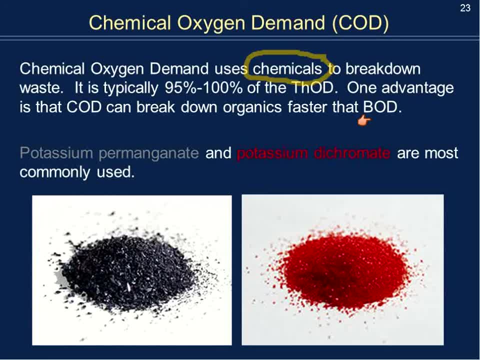 If you don't have to add additional chemicals, if you can grow and maintain good bacteria or good organisms, then you have your source. You have your source that will break down your waste for you. But it's a better choice to say that the chemical oxygen demand turns out to be 95 to 100 percent. 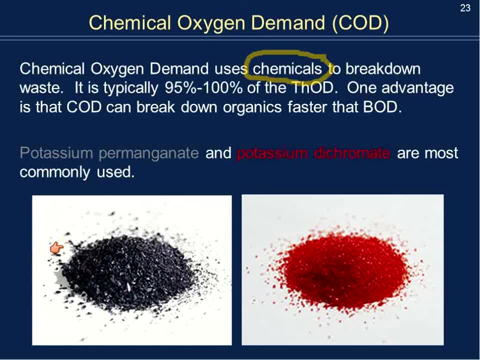 of the theoretical oxygen demand. So there's a number of reasons why you need to go through the process to see whether the chemical oxygen demand turns out to be 95 to 100 percent of the theoretical oxygen demand. The second way to do that is to catch a dellucan. 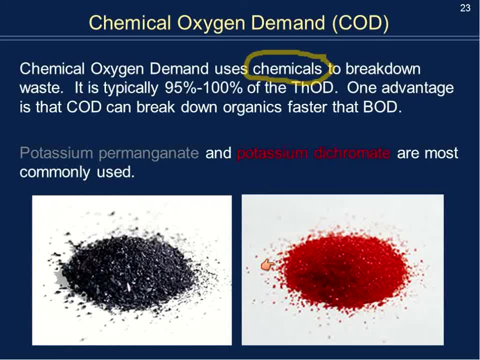 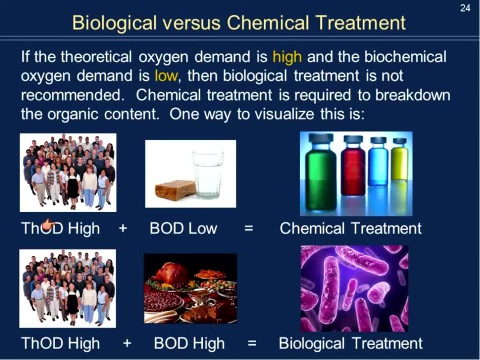 So a kettle to a wastewater treatment system to break down your organic matter. The question should be: well, which method do you use? Do you use biochemical or do you use a chemical treatment? It depends on what's available If the theoretical oxygen demand is very high, meaning that you have a large amount of organic. 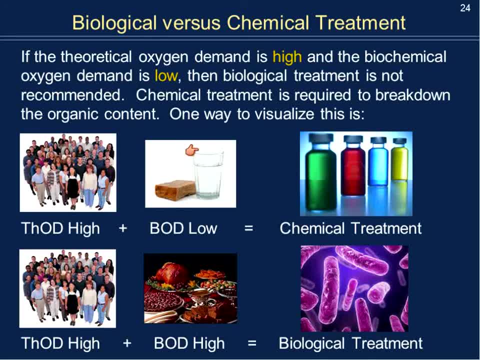 material, however, there isn't a lot of oxygen available, So again think that there's really nothing to break it down. then that means you need chemicals in order to break down your waste, where instead, if it's calculated that the theoretical oxygen demand is high, meaning there's a lot of organic material to be broken. 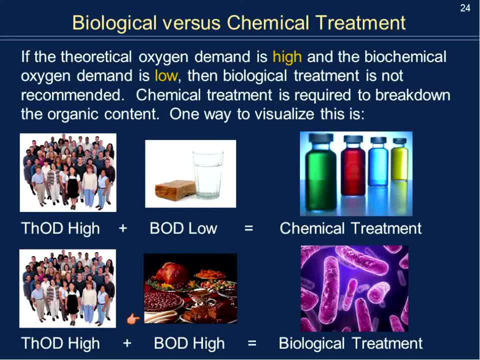 down and there's a large amount of oxygen present, well then you can use biological treatment. That's often how it's chosen. So very often we use the theoretical oxygen demand to determine what we need- How much oxygen- And then the, depending on your system, whether you have available to you a large amount of. 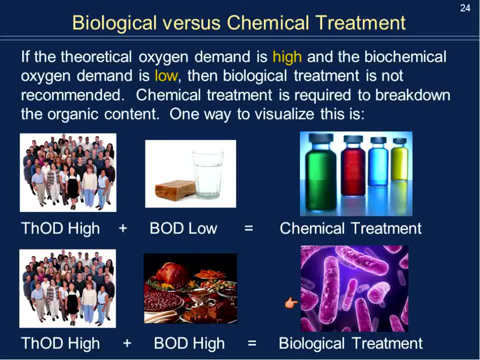 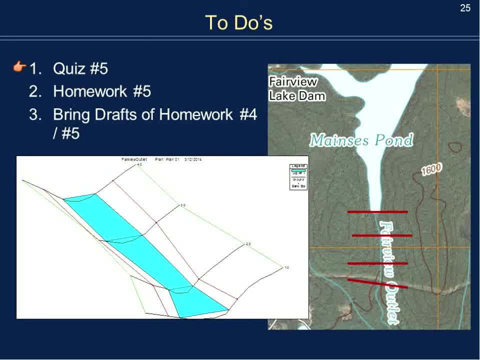 organisms that can break it down or, if not, you use chemicals. So that brings us to the end of our objectives. So what do you need to do? Please make sure you do quiz number five before the deadline. Please review and start homework number five, which is your HEC-RAS model.